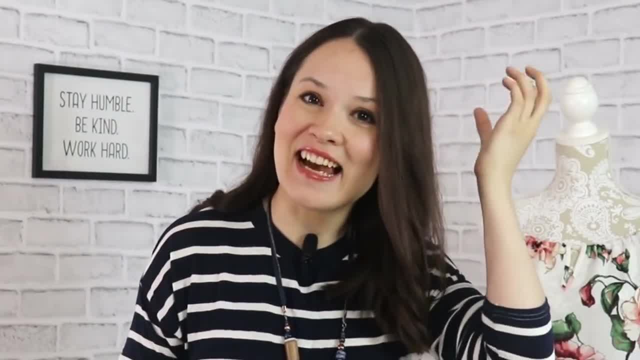 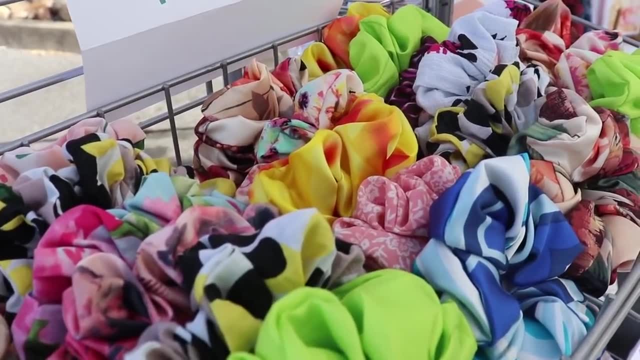 it doesn't pop, it stays together, nice and tight on my hair, just like I like it, and it's such a pleasure to wear it. So when people come to my booth and they're like, oh, these are scrunchies, I share with them this personal story of how I came to make these scrunchies for myself. 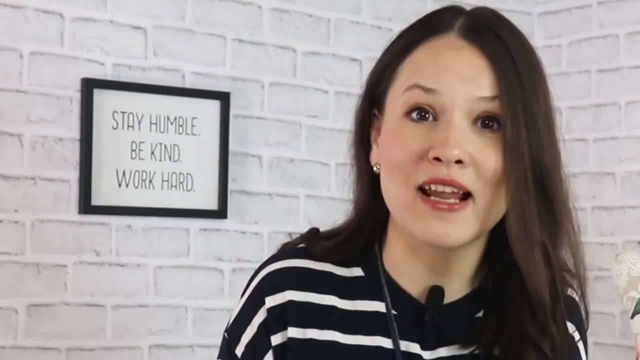 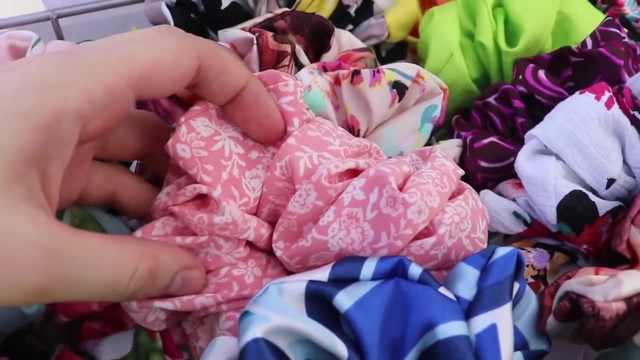 and then I realized that a lot of people might have exactly the same problem that I do. So that is one of my unique point of sales. I tell them you're more than welcome to grab it and you will feel that white elastic really supporting your hair, especially if it's on a 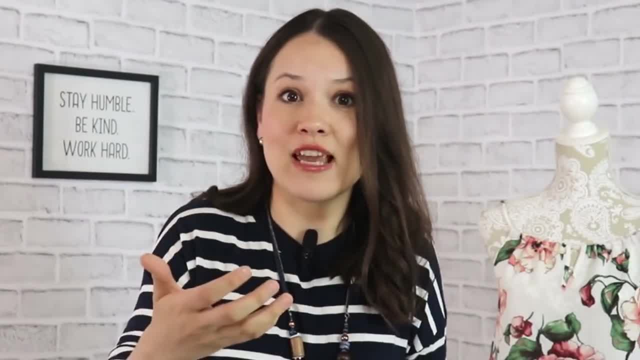 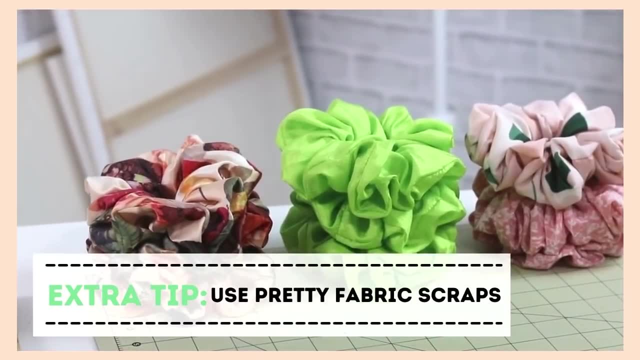 side. So I share with them my story, my personal struggle, how I overcame this, and it doesn't have to be a long thing. And then I also make them from really fun colorful fabrics and materials and I use my scrap fabric for that and, believe me, I have a lot of really fun scrap fabric pieces that make. 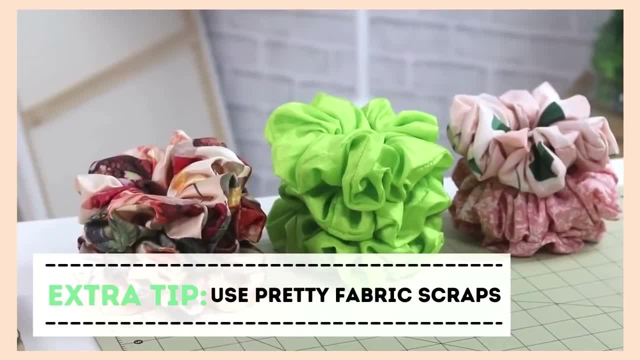 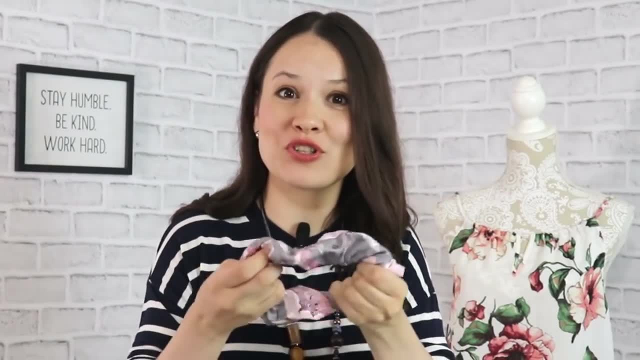 this huge fun assortment of scrunchies for anybody to choose what they really like. And here's an interesting thing: Oftentimes, once people feel my scrunchies, they'll purchase two or three, sometimes even four or five at the same time. And that's because scrunchies are so easy to make and it's 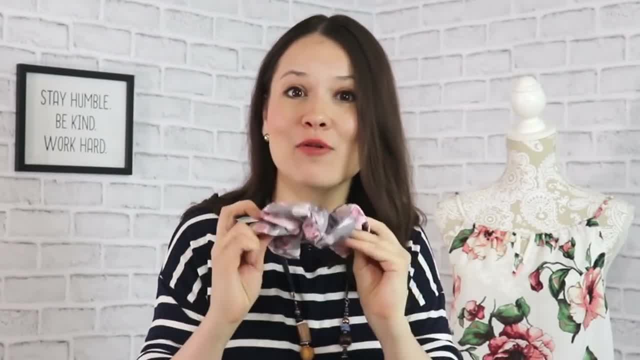 so easy to make. So I share with them my story, my personal struggle, how I overcame this, and it doesn't have to be a long thing. And then I also make them from really fun colorful fabrics and materials at the same time, because they really love how it feels and how it looks. Now another really 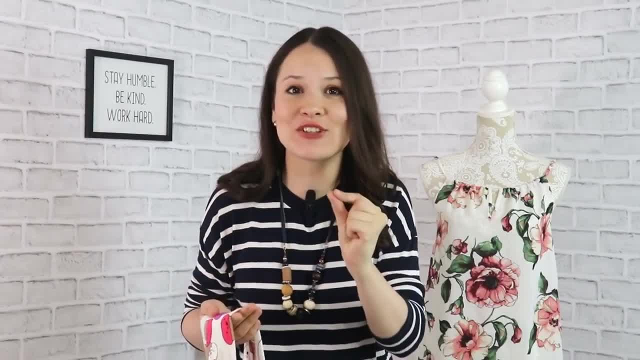 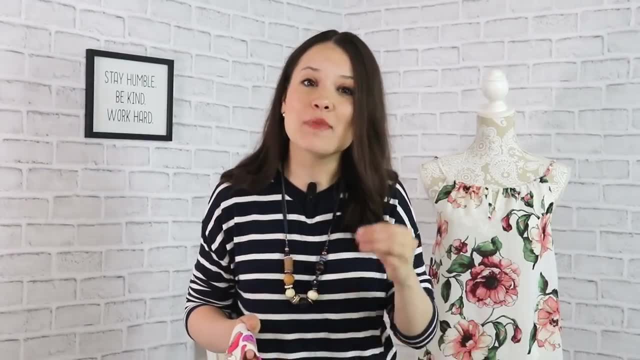 important thing that I've learned by doing this farmers market is to listen to your guests. to listen to your customers when they come to you in person at the farmers market- or that might be online as well- because they will tell you what are they looking for, what are they craving and what. 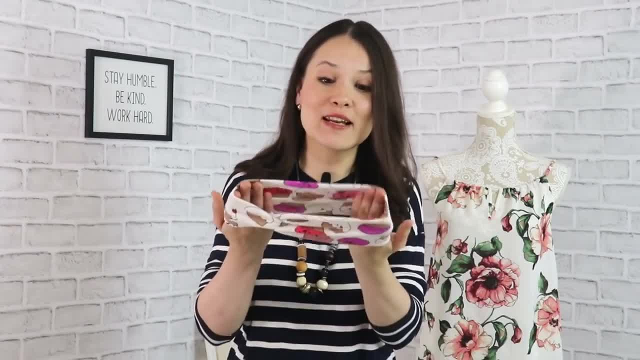 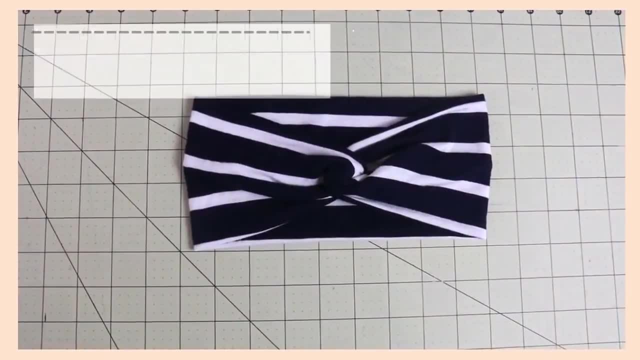 are they willing to spend their money on. And for me, one of those items was headbands. Guess what? on the first day of the market, people kept asking for headbands. they kept asking: well, do you have any pretty headbands for me and for my granddaughter, or for me and for my daughter? 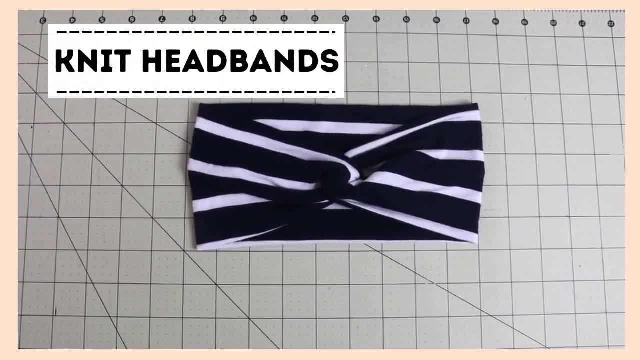 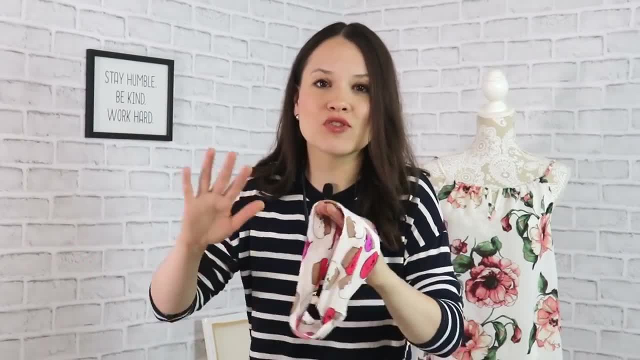 and I didn't. I started my farmers market with three simple initial items to sell for a variety of reasons. I was just testing the waters. I didn't want to make so much inventory that would sit without being sold. I also wanted to see what people would be excited about. 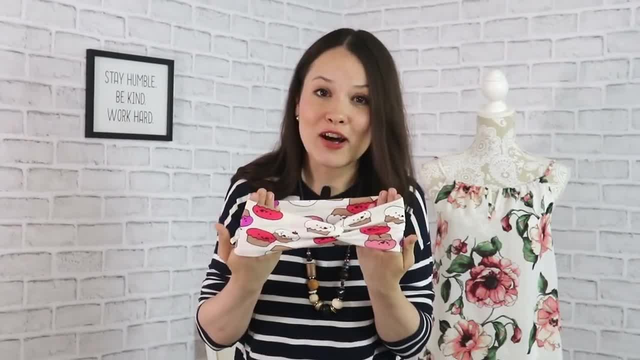 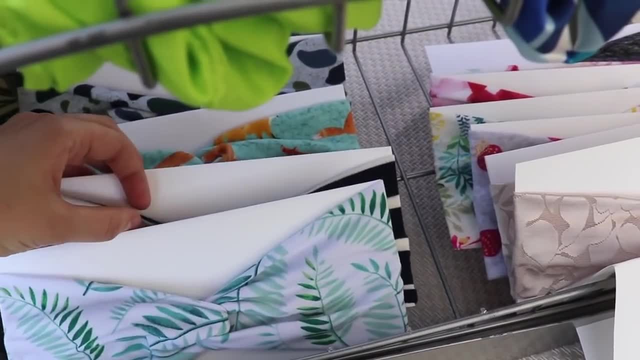 and guess what? headbands was one of those items. So I thought: definitely for the next farmers market I gotta make some headbands. Besides, a couple of weeks before that, I did a really fun video about using your knit fabric scraps and one of the items was to make 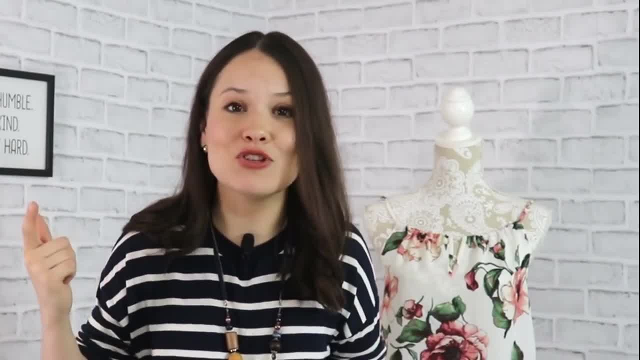 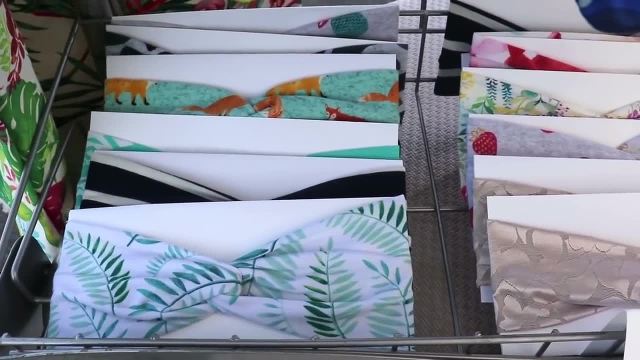 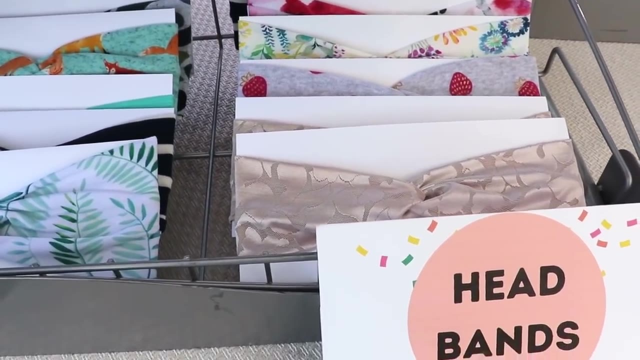 a knotted headband like that, So it was a win-win. I already knew how to do it. I had plenty of gorgeous, fun, colorful knit fabric scraps that I could use to make these really fun headbands, and the response was great. People kept saying that these are really nice and soft and they fit your. 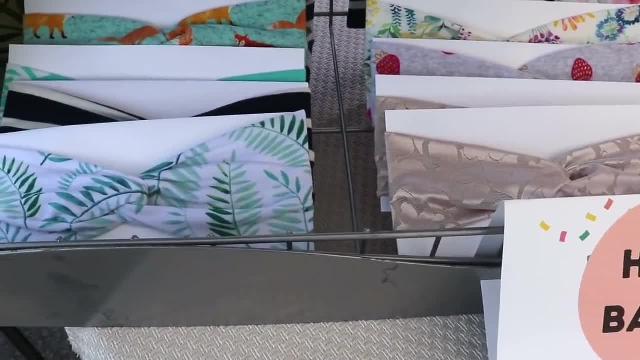 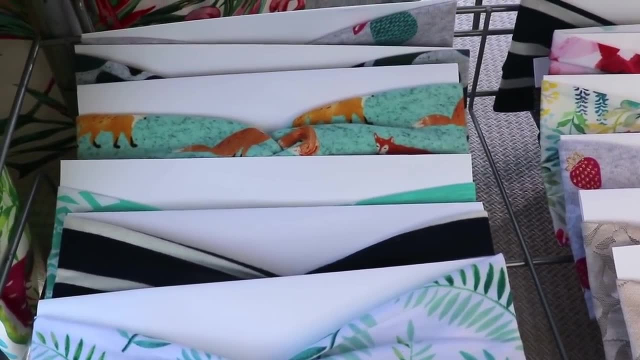 head nicely and people kept purchasing them, sometimes two or three at a time as well, So this is definitely one of the items that, based on my experience, should do pretty well, no matter where you are, And also one of the unique point of sales for this item is that I mentioned that. 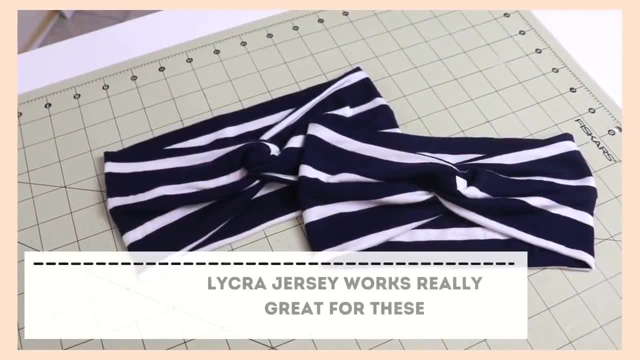 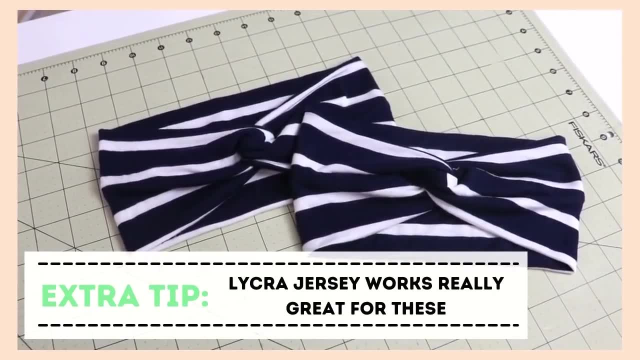 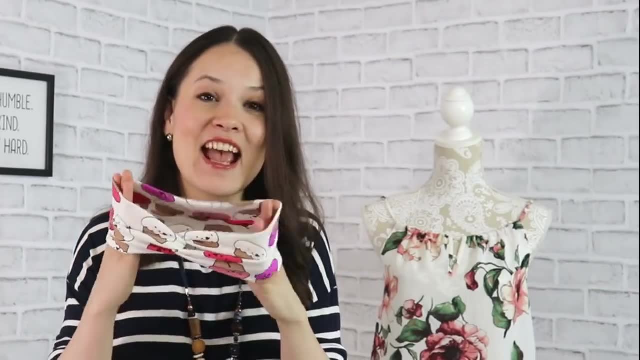 during colder times, you can use it as your ear warmers and that's another thing that you can put aside in a note for yourself that if you do participate in winter time farmers market, you can make these out of warmer materials, like really nice knit or really nice thicker jersey, and use. 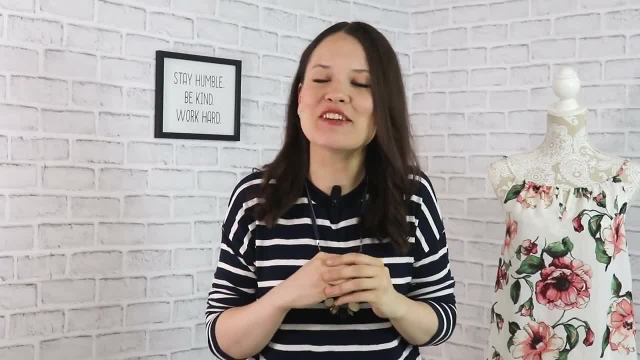 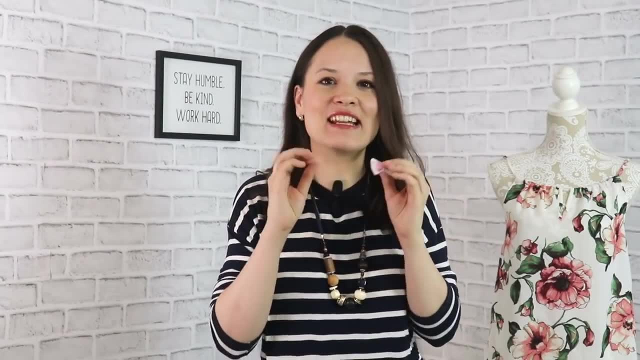 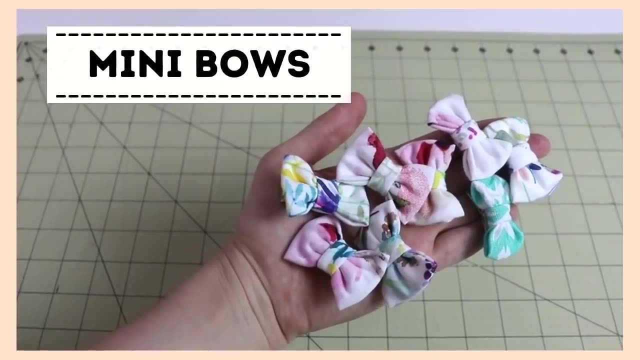 these as ear warmers. You might not know this, but we live in a really small town, so the size of our farmers market is really humble, and, with that in mind, I wanted to create an item that would cheer up anybody's day, no matter how big or how small is your budget, and one of those items is this cute little bow. 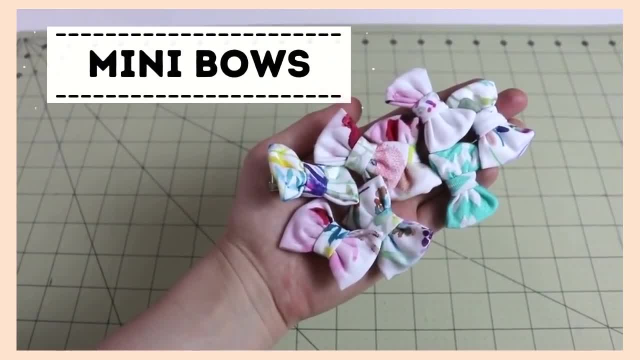 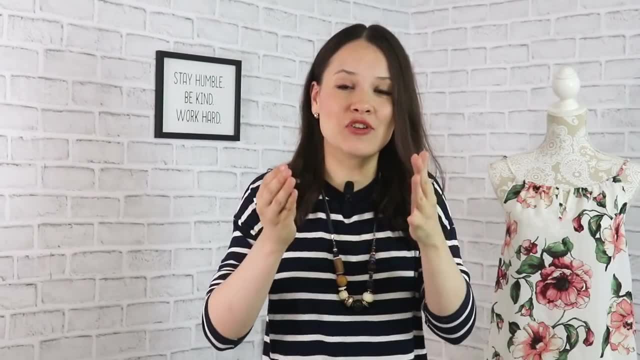 It's a clip that goes in your hair, usually geared towards younger children, but how cute it is, how easy it is to make and, as I said, it will cater to any budget size, whether it's smaller budget or larger budget. And I also, as a parent, know one of those moments when you go somewhere. 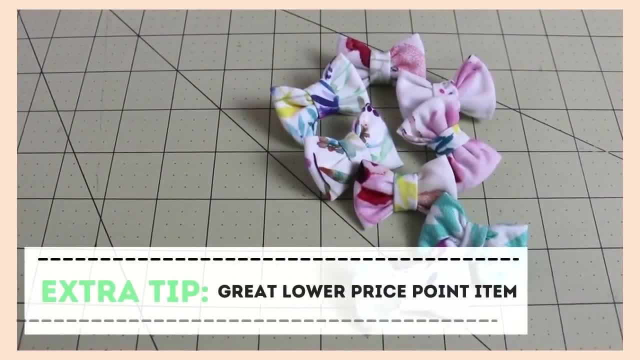 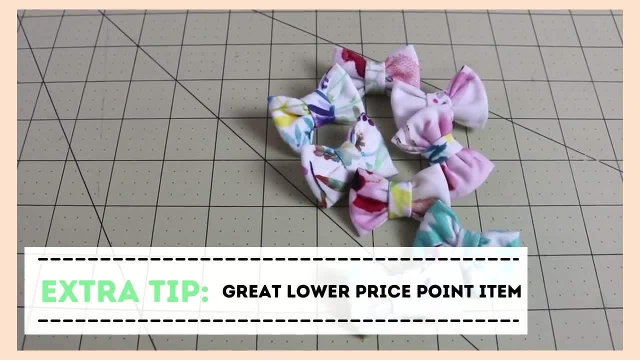 and your kid really wants you to buy something, but maybe your budget is limited and you want to make your kid's day but you're unable to buy something that costs double digits. but this little one anybody can buy, even with the money that a tooth fairy left for your kid. 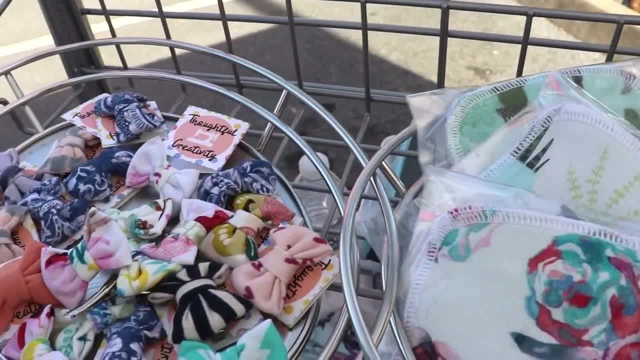 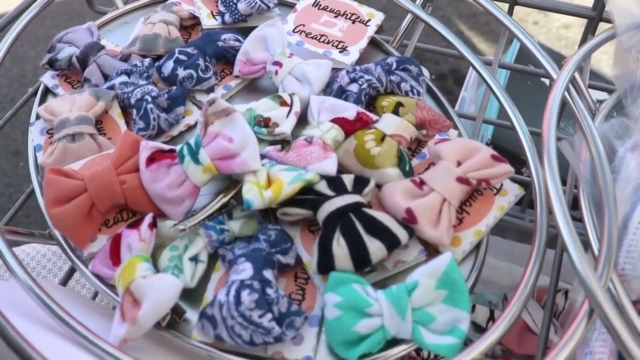 Now, do you see these cute little tags that I made for these little bows? It's adorable, isn't it? Now, that's one of the things that I wanted to talk to you about. From my perspective, it's great to have, but you don't want to go overboard with it, so that way, it feels less and less handmade, and that was. 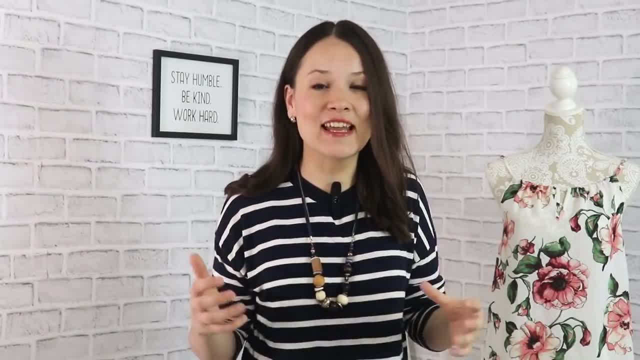 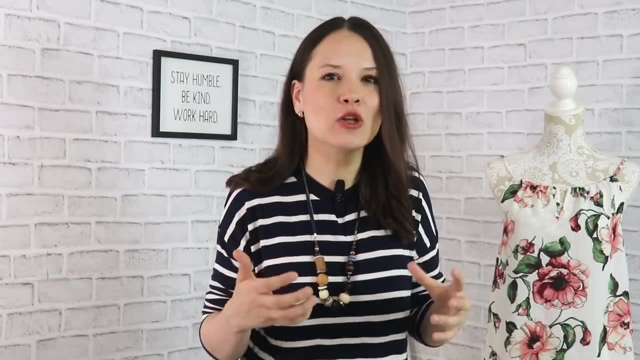 one of the challenges that I faced. At first I had a lot of tags on a lot of my products, but then I realized that people were really questioning whether that was handmade or not, just because it looked more like store-bought product. so I definitely scaled it back a little bit. but if 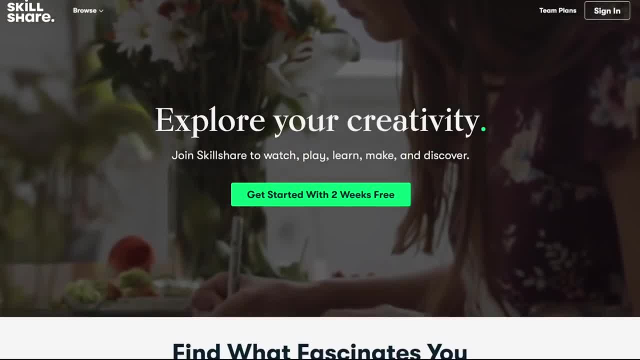 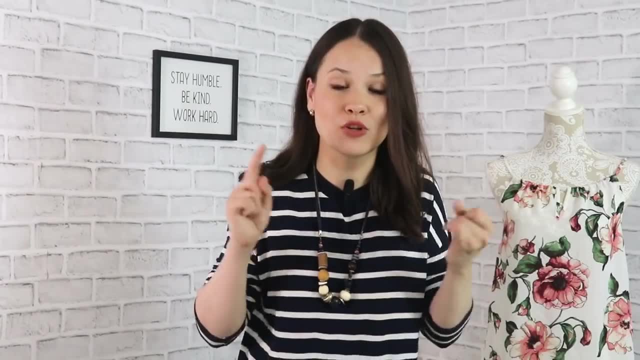 you're looking to sell some of your handmade items. that's where Skillshare comes in. It's a learning community with thousands of classes on different subjects, and some of the subjects are things that are there to help you out with your personal branding, with the branding for your business. 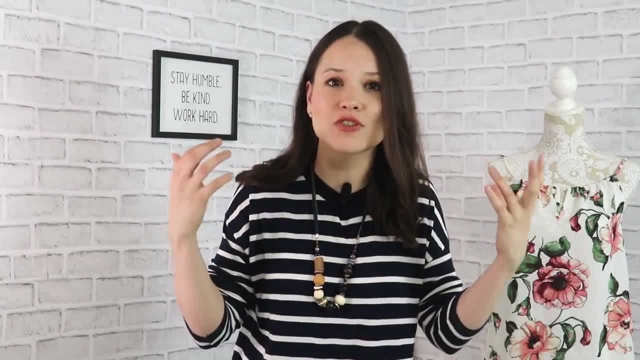 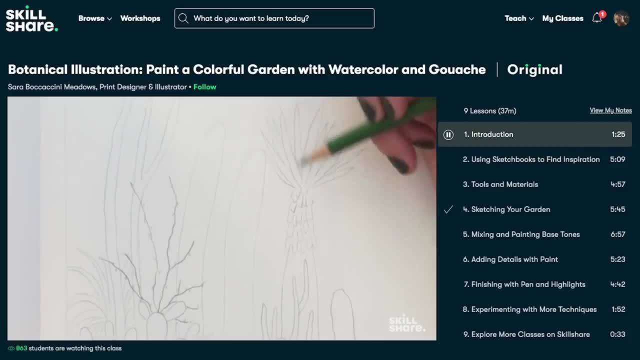 with some of the ideas- how to build your business or maybe your influence online- and it's a great place where to try new hobbies and new creative things and ideas. I've been a Skillshare member way before we started working together and my go-to topics 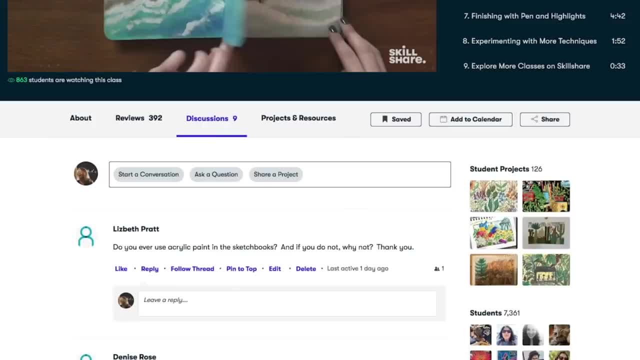 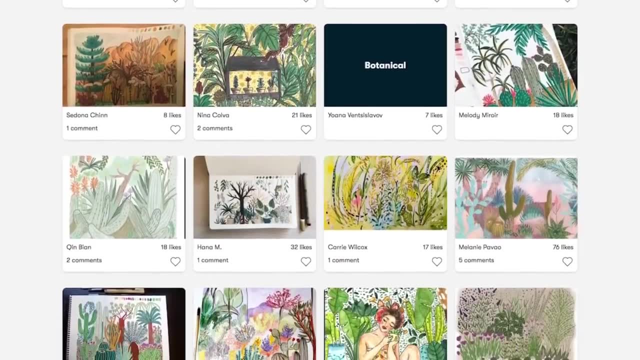 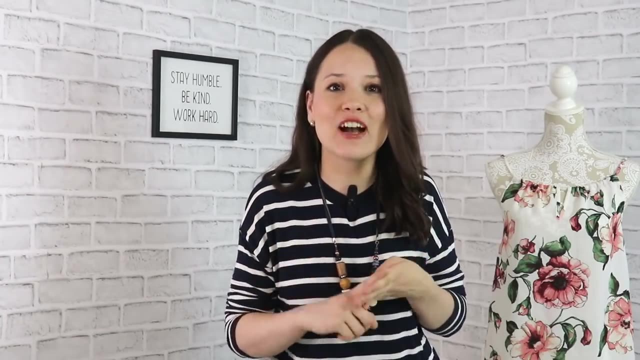 when I log in onto Skillshare are watercolors, sketches, illustration and also productivity and sometimes some of the photography tips and tricks and knowledge for my YouTube channel. Now for you are some amazing classes on topics like lifestyle, photography, productivity, fine arts, creative. 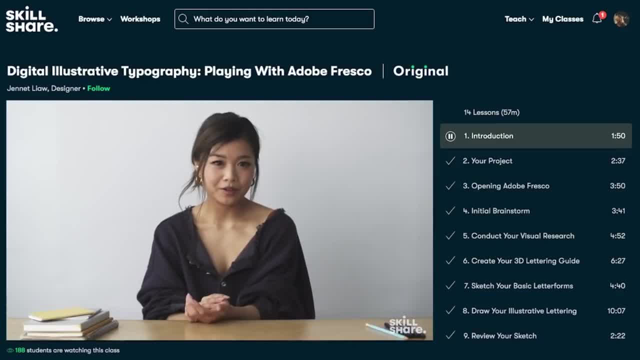 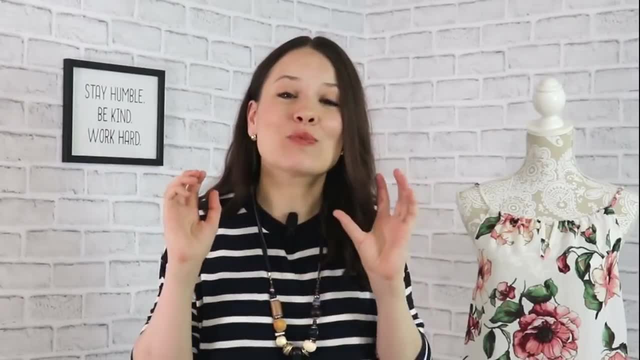 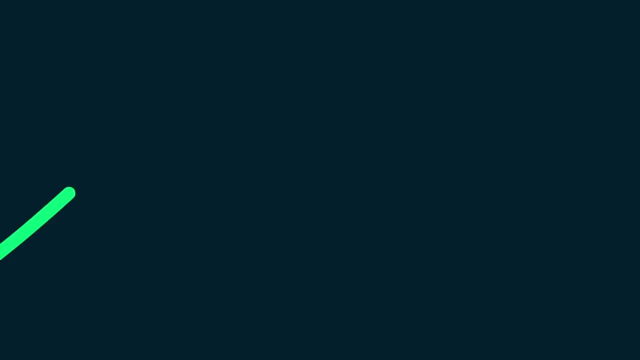 design and many, many more and for 1000 of first subscribers. to click on the link in the info box below, you will get a one month free of Skillshare premium membership to take it to try it and see what it does for you. There's no ads, it's centered around learning and it really is a great place. 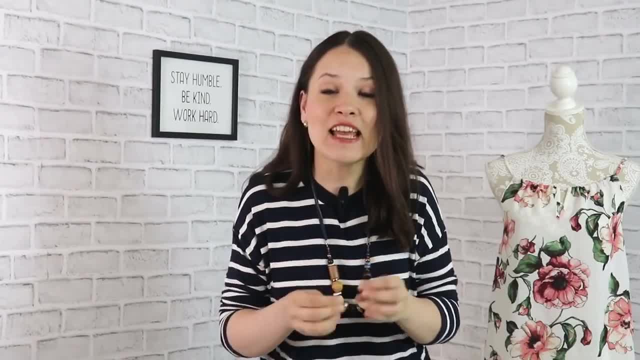 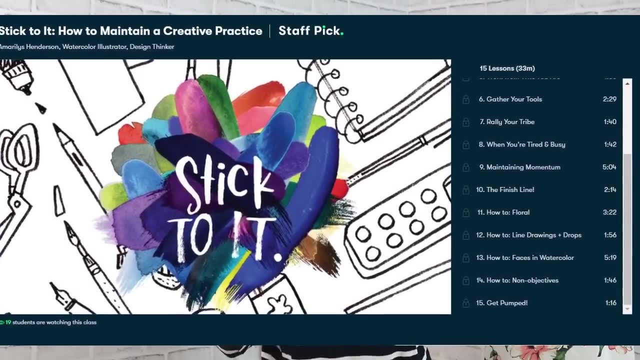 where to learn something new and just hone in on your creativity. and for me, currently I'm looking at this class by Amaryllis Henderson and she is talking about how to stick to your creative practices, how to really follow through with your creative ideas and your creativity. 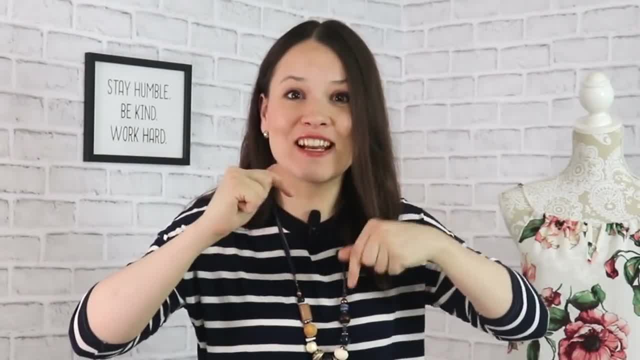 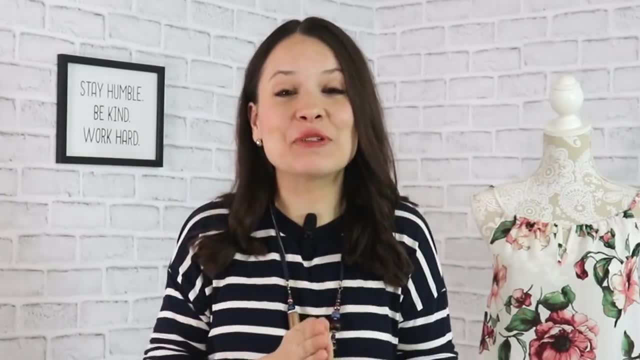 all together. So definitely check out the Skillshare offer in the info box below and let's roll with another handmade item that I sell at my farmer's market. Now this next item I actually received as a gift this last Christmas and I really loved it. 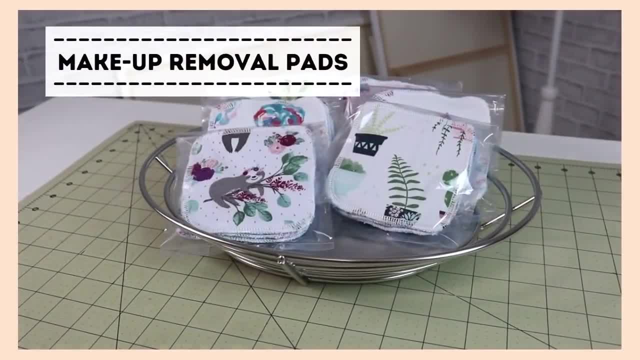 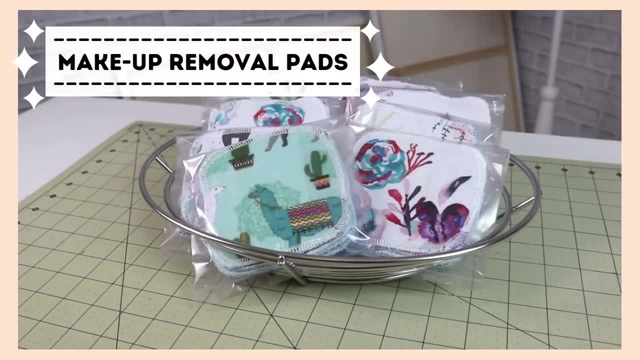 I use it all the time and I thought, well, if I love it, a lot of people out there will love it as well. so I decided to try and make it and see how it goes. and those are makeup removal pads. I sell them in a set of five. they come with one side in cotton and the other side in this toweling. 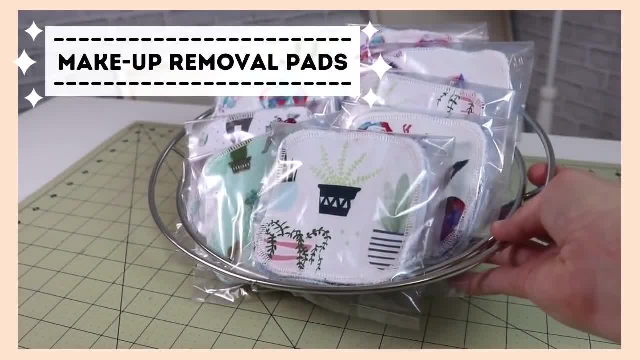 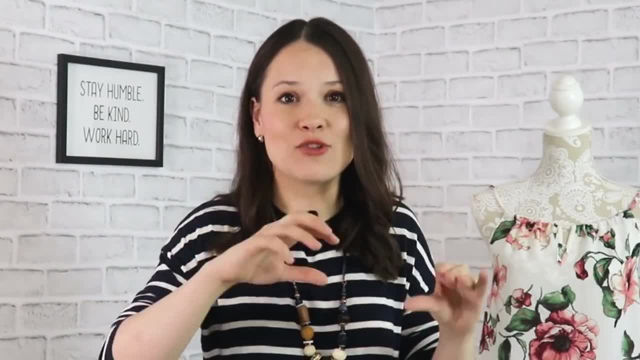 material, so that way it exfoliates it really nicely, and I need to tell you that they are a winner. People love them. The only thing that I've noticed- since this is a really new item that I've added to my farmer's market only two or three weeks ago- is that a lot of times when people 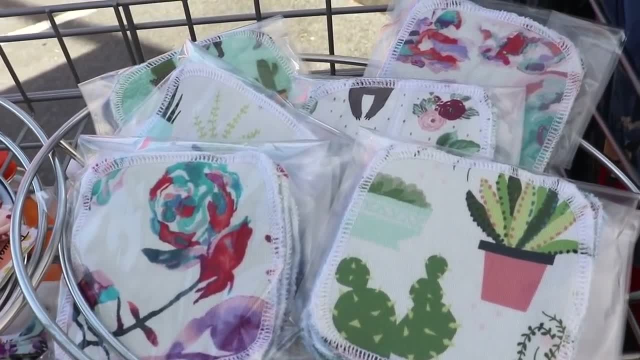 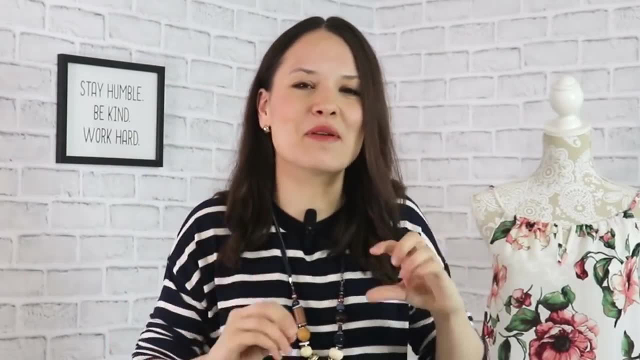 pick them up. if I'm not there to talk to them and chat with them about what is that we're going to do doing here and what is the purpose of this, then a lot of times people think that those are coasters. So I definitely need to do a little bit better, maybe with signage. 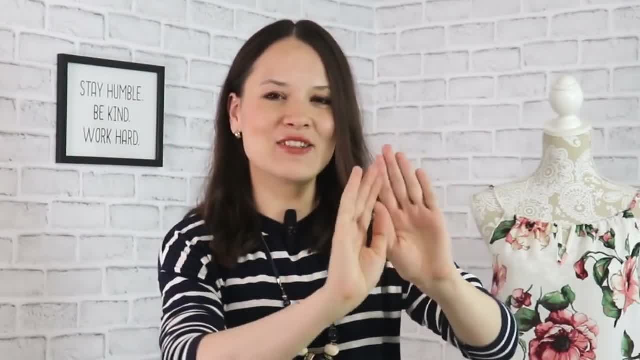 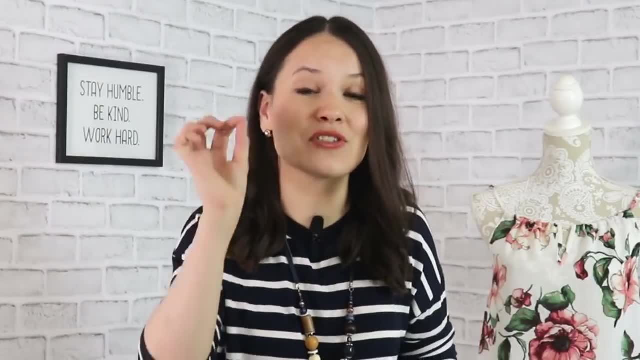 maybe with some other marketing materials that will point them into the direction that these are makeup removal pads and not coasters, Although if people pick them up and they think that those are coasters, this is another tip for me to think that, okay, maybe if I do make some coasters, those 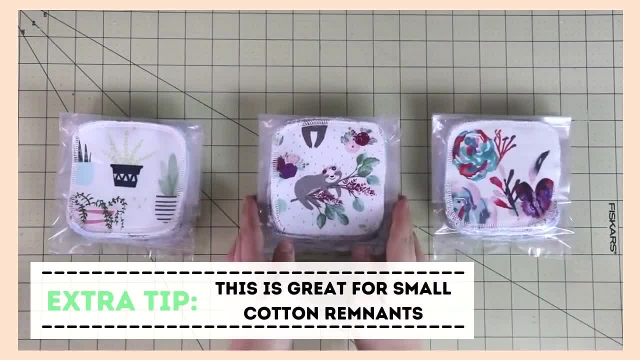 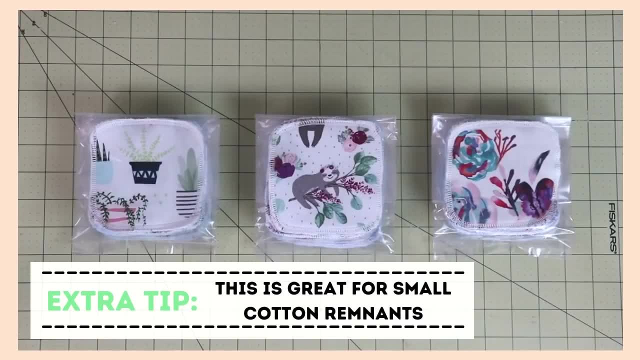 would sell well as well. But either way, these are really fun makeup removal pads. people love them. I packaged them up so none of them are loose. People can't actually touch them, and that was one of the things that I was really concerned about: thinking that well, if people can't touch them like they can't touch. 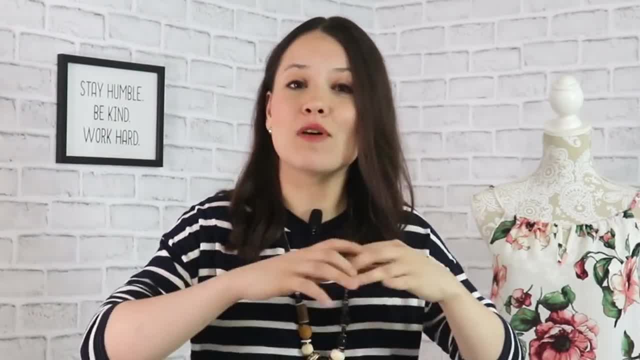 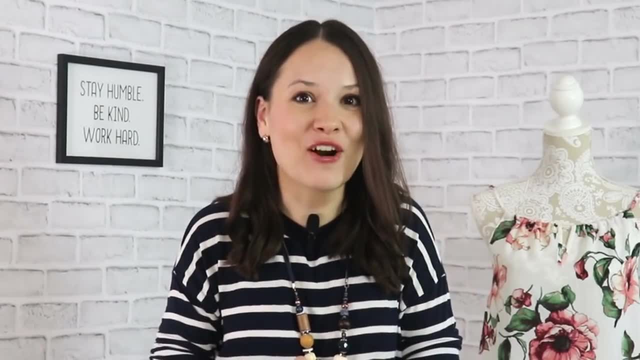 scrunchies or headbands. maybe they're not going to buy them, But it was no problem whatsoever. People grab a little set, sometimes two at a time, and they purchase them and so far the feedback has been amazing. Here's another item that is a very recent addition to my farmer's 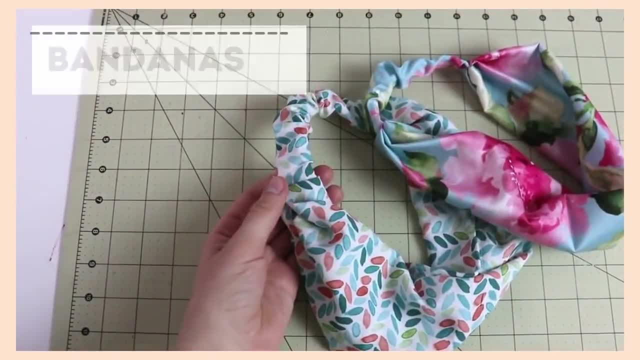 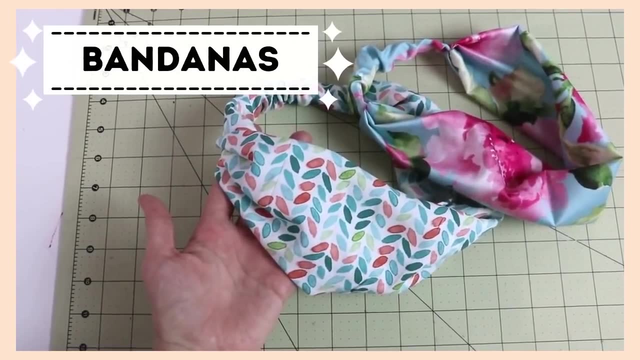 market inventory, and here is another lesson to learn. I've only made two, and I can see that people are excited. they pick them up, they look at them, they ask questions, but there's only two, so there's nothing to choose from. Therefore, make more than just a couple. 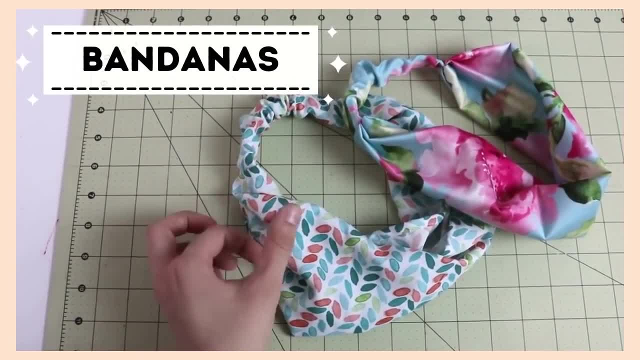 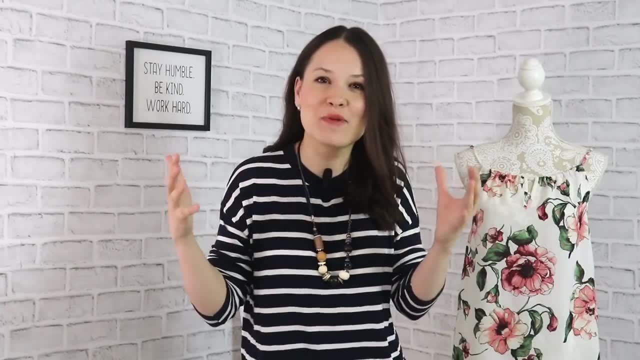 Make a variety of items of the same item in different fabrics or different prints or in different colors or whatever else that might be, because then, when there is a choice, people are more likely to find what they're looking for or maybe what suits their taste. So these are. 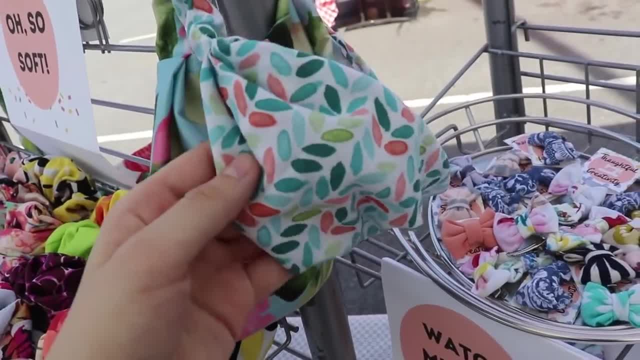 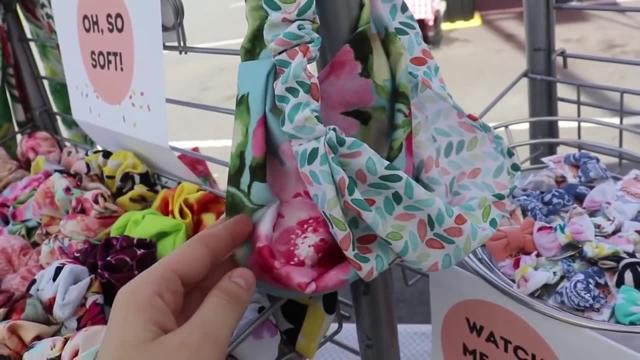 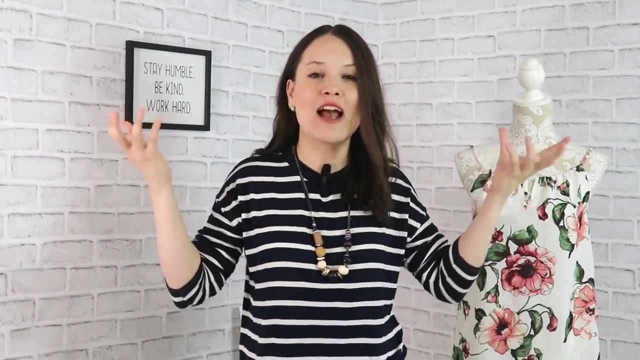 actually bandanas. They're made out of woven fabric and it looks very similar to the hand band that I've showed to you before, with a twisted front, but these are just made from woven fabric and they cover more of your head, so it kind of acts like a sun hat or a bucket hat, but without. 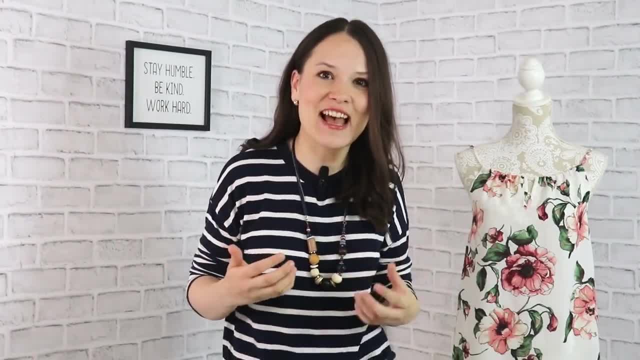 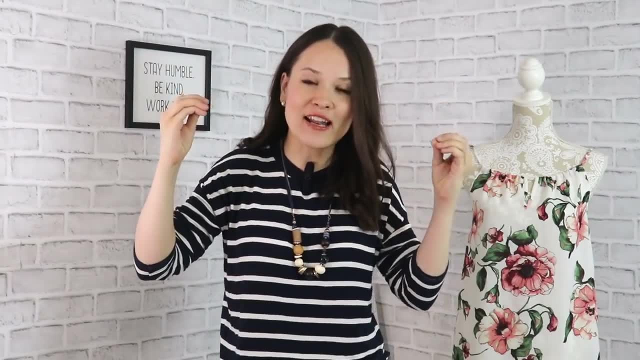 actually wearing a hat. A unique point of sale here is that if you are working in the garden and you like to wear your hair in a ponytail, if you put a bucket hat on, you actually can't really put it on that well, because that that ponytail is going to stick out. So these would be really great. 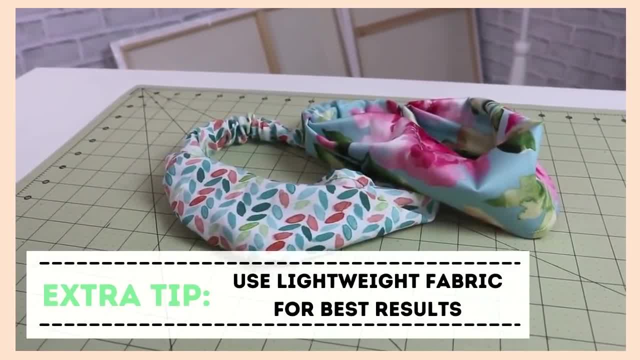 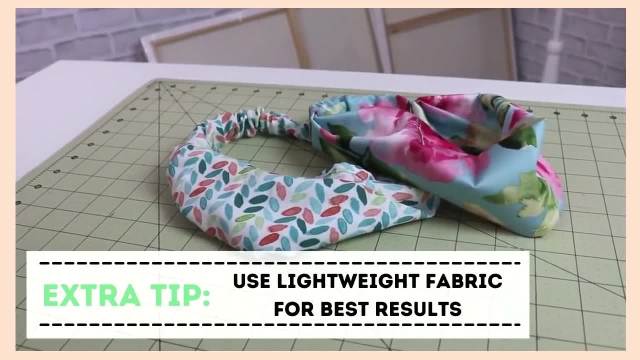 because they do cover a lot of your hair. So if you're looking for something that's really from your forehead all the way to the back of your head with elasticated back, but then you still have enough space for your hair to be out and to be gathered in a ponytail, So I definitely need to. 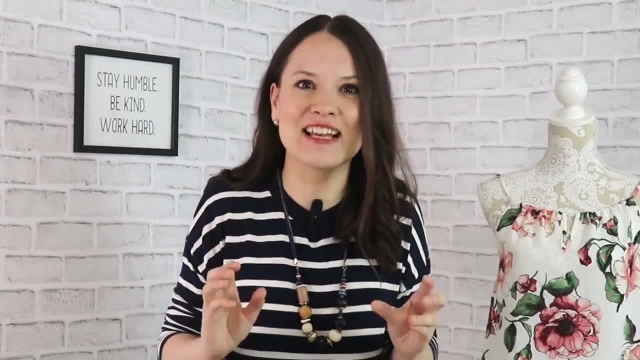 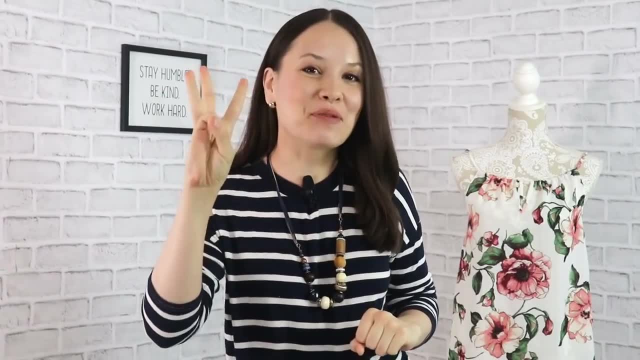 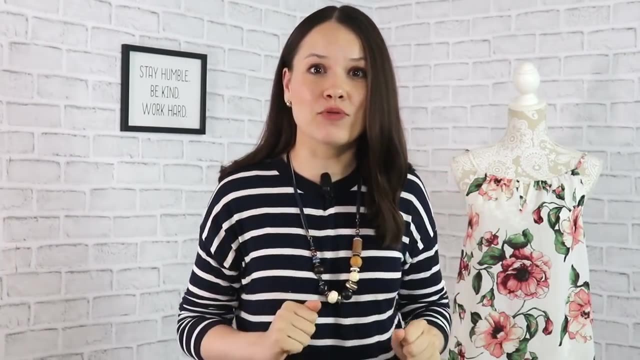 make more of these. I was in such a time crunch last week so I only made two- My bad, So I definitely need to make more and see how it goes this following week. I have three more items for you guys to discuss in this video, but before we do, I wanted to remind you: do your research before you apply. 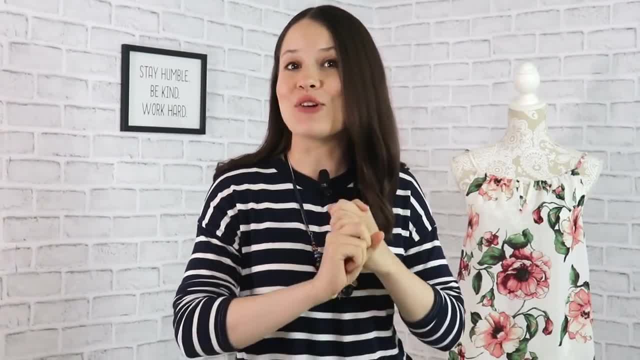 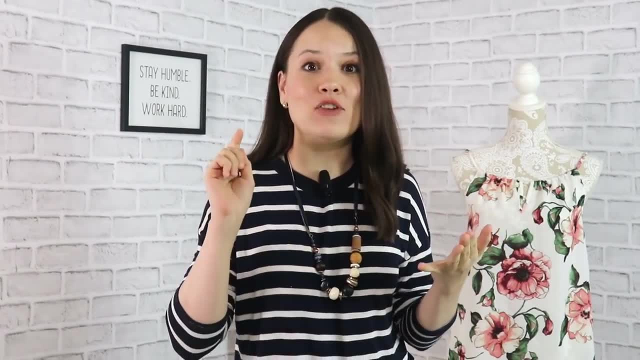 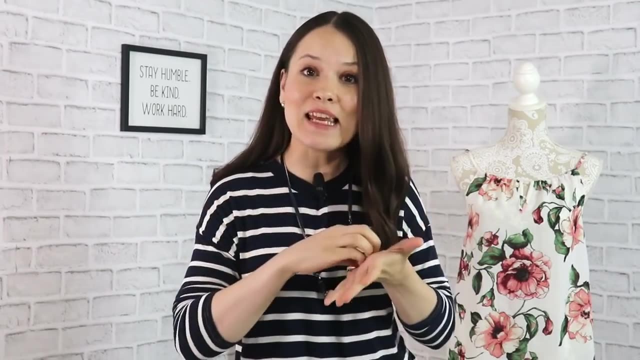 to a craft fair, farmer's market. before you sell online or any other business endeavor, Take a look if there are any regulations that you need to know about. Take a look if you need to submit your items to be inspected. Take a look of how big or how small parts need to be. Do you need any labels? 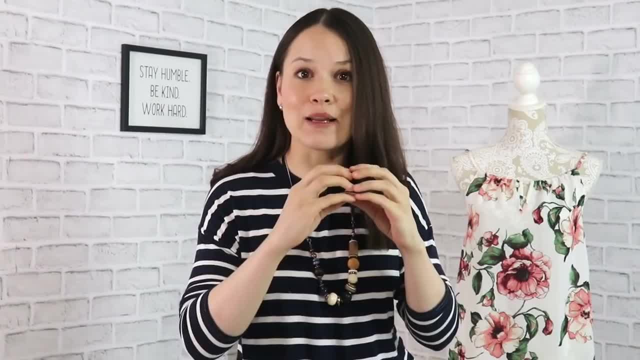 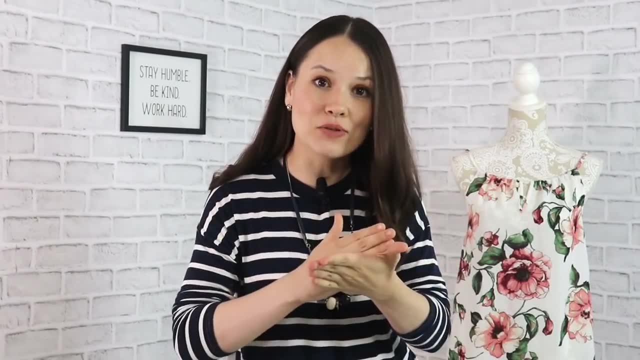 for those particular parts or if you're selling smaller items. Don't skip this step. Be resourceful. Right now, you can access information easier than ever. Everything is at your fingertips, So definitely do your research, Be resourceful And make sure that everything you're doing is according to the local regulations. 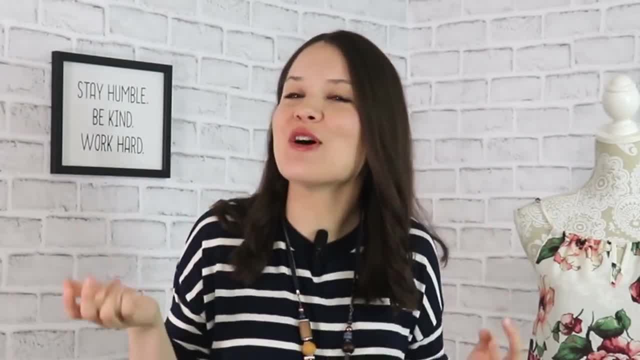 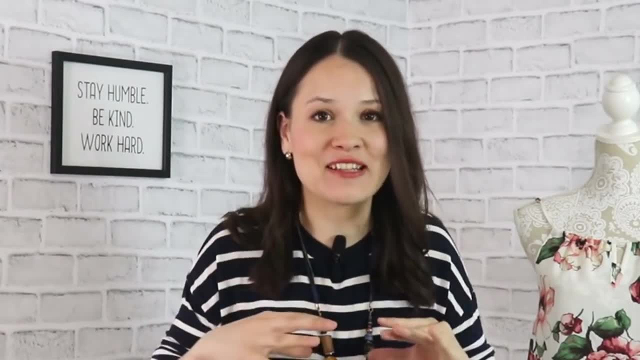 Now, if you're watching this video and you're thinking, well, I wish you would actually show how to make these things. Well, dear selling friends, all the tutorials for all of the items that I mentioned here will be in the info box below underneath this video. So definitely, 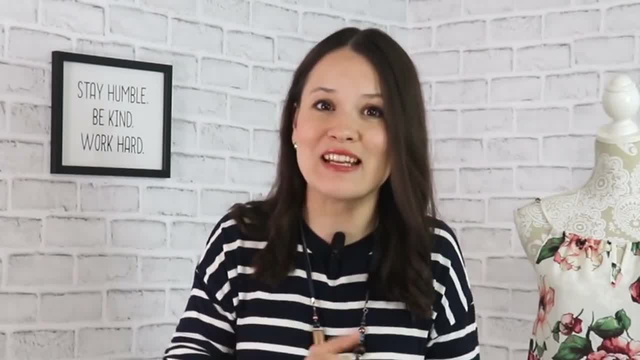 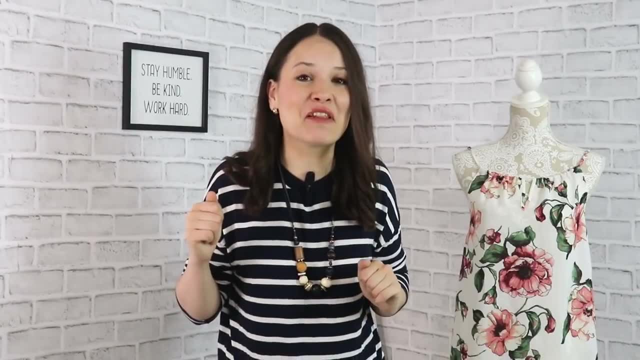 take a look over there. It's sorted out. Everything is noted for your convenience, And if you've been following me for a while, chances are you've already seen it. If not, if you're new here, well, today is the day. You have a lot of really fun videos to look forward to, and 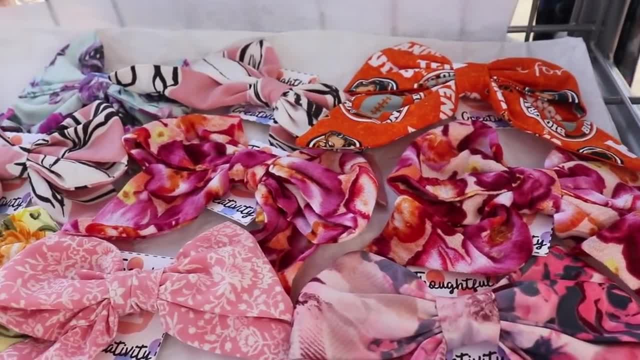 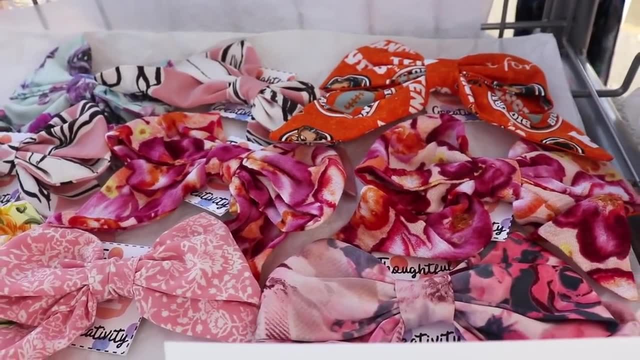 check out the info box. Now, this item. I really thought it would be such a great idea, truthfully, and partially because I like a really pretty large bow on my child, Although it never stays in because she just takes it out. She's two and a half, so she can't be bothered with having anything. 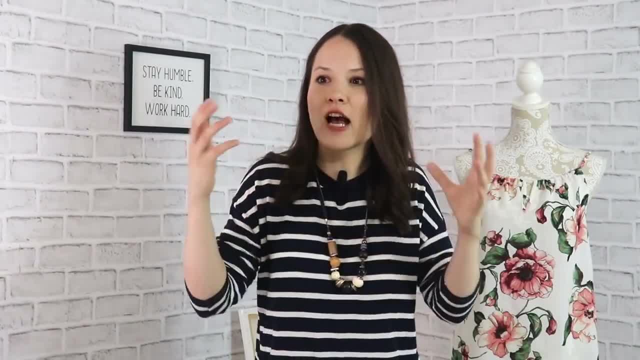 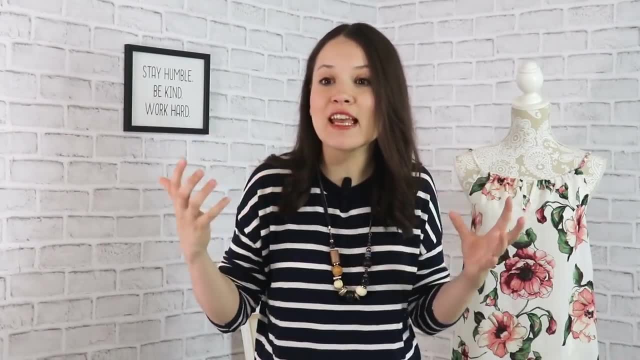 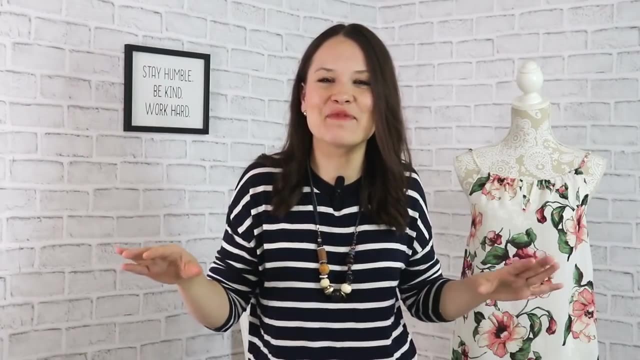 in her hair. But I thought: well, definitely, especially in our area. cheerleading is huge, Sports are huge. People are going to love these. They're going to buy these for their kids And absolutely no The worst selling item out of the whole lineup of whatever I sell at the farmer's market. 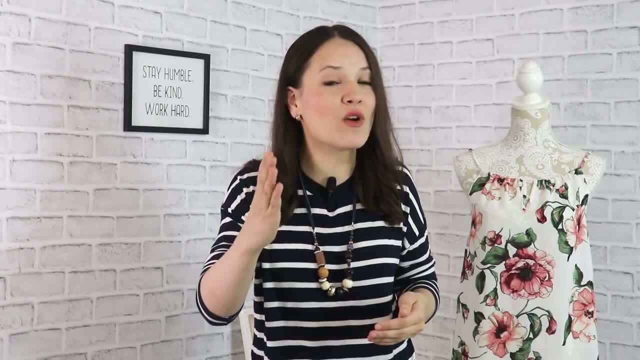 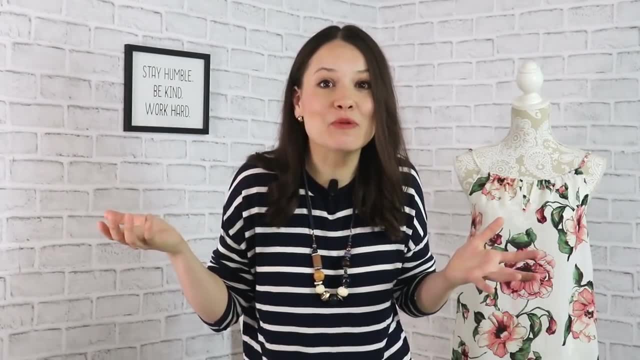 So this one has been definitely a fail. It might do really well in your area, Who knows? But in my area, for whatever reason, these large bows just don't interest people. Here's another really useful tip that I've learned, not necessarily from this farmer's market. 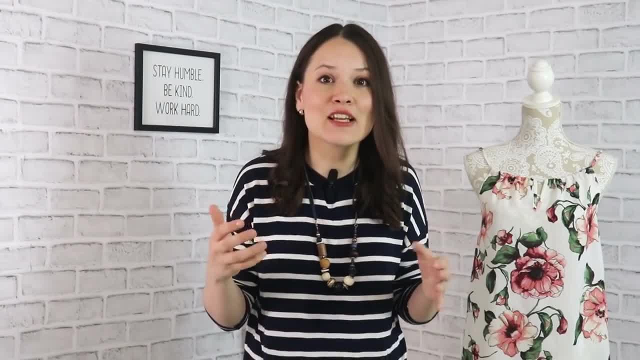 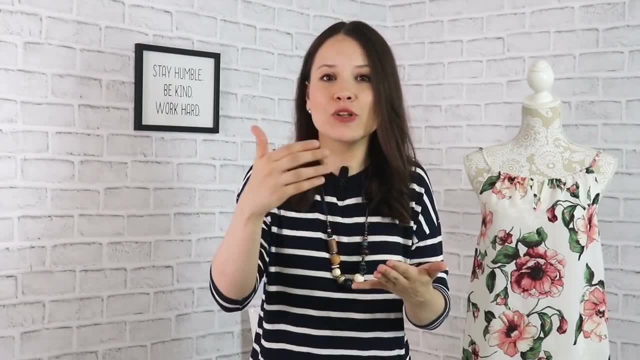 but more from all of the years of my professional employment. and that is to really analyze not only the price that you want to set for your items and for your handmade goods, not only to think about what are the resources- time- and what are the materials. 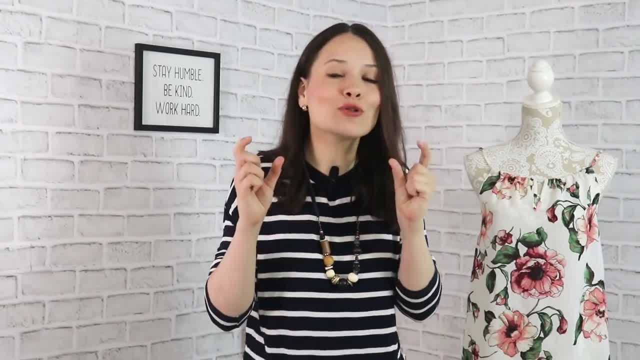 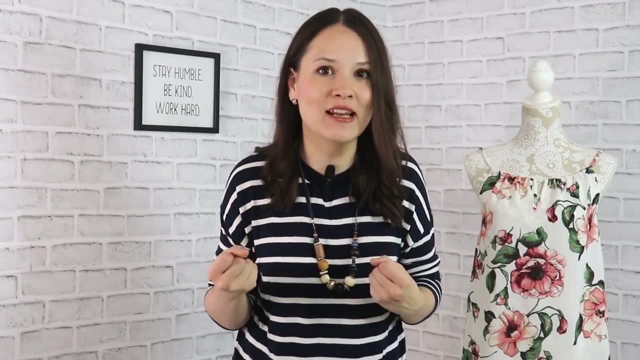 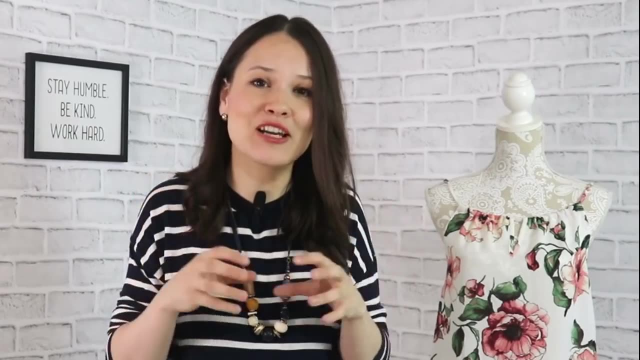 and equipment involved in creating this or that item, but also what is the purchasing ability of your target audience. How much can they actually spend on your handmade item and will they spend that money on that handmade item? As I mentioned, we live in a smaller town and our farmer's market. 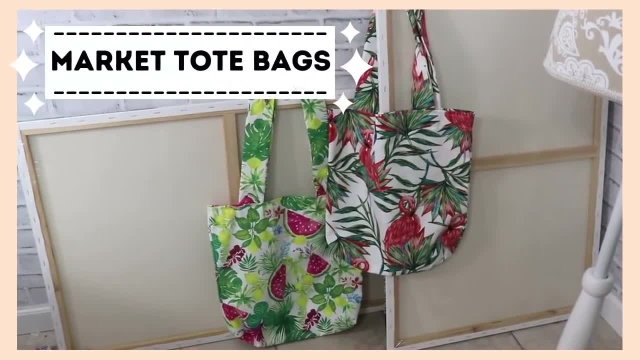 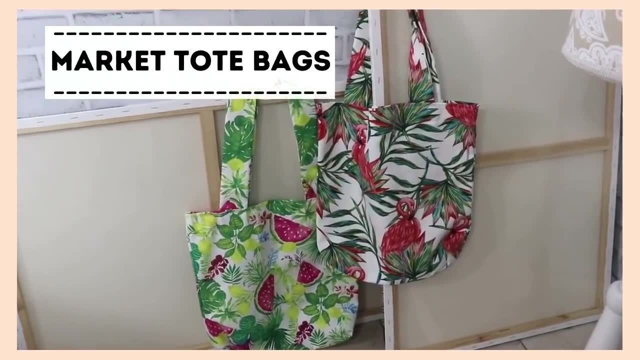 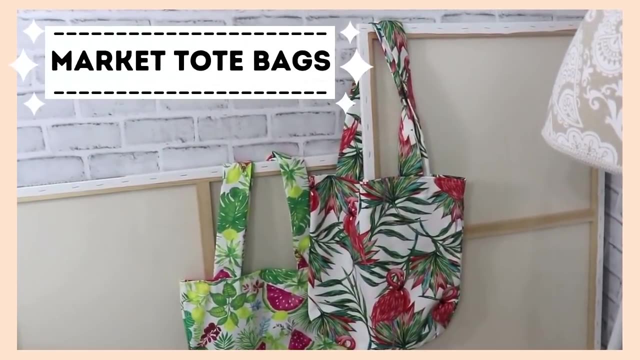 is of a very humble size. So I made these tote bags and I truly think that they're fun, They're awesome, They're colorful. The main idea here is that you can buy these bags in the market. You can buy them everywhere. This is one of my favorite bags. They're so cheap. You can buy them. 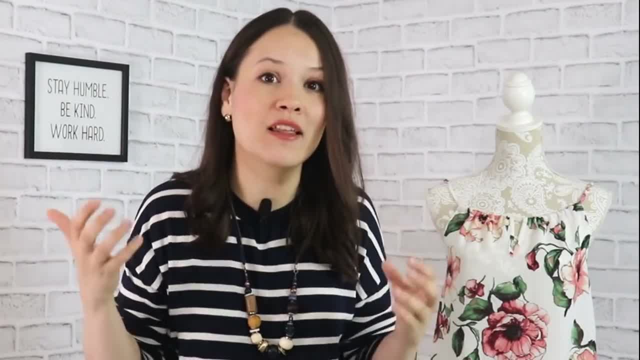 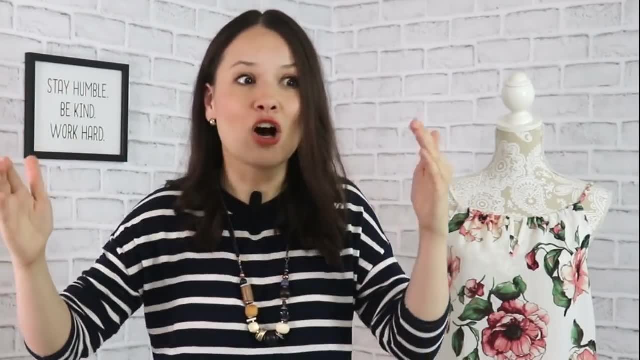 at any store. I actually like the name. It's made out of a really nice sturdy fabric. I actually use outdoor decorating fabric for these and that makes them really nice sturdy. They don't sag when you put stuff in them and I truly think it's a really fun, nice, quality item. However, because the fabric is so expensive. the tote bag is at the more expensive end of any other tote bag offered on the market. Therefore, when people look at them, they're excited. They're like, wow, this is a really nice tote bag. They will ask: how much is it? I'll tell them. 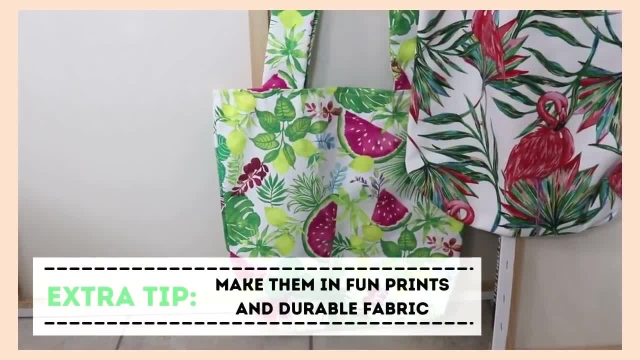 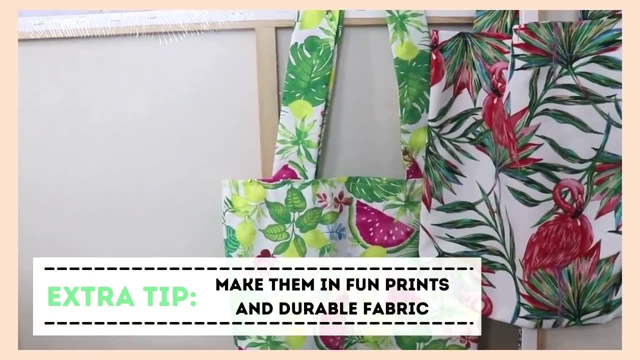 the price, And I could see that they're not ready to pay this much for a tote bag. So here I definitely encourage you to think about the purchasing ability of the target audience in front of which you're going to be selling, whether that's online, offline or in any other way that. 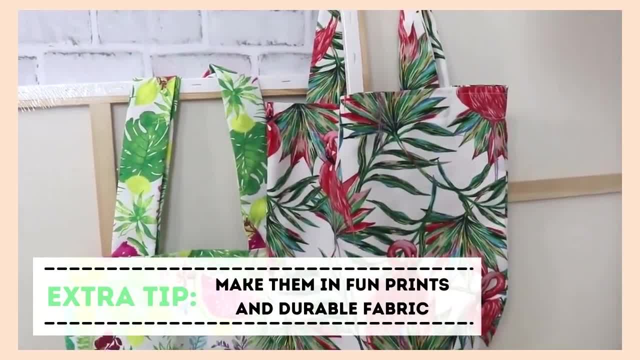 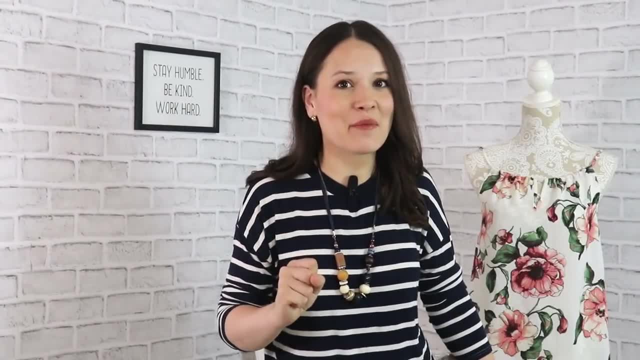 you are selling your product. Think about what are they able to purchase and what is a good price and a good item for this or that market. Another really good thing to think about is seasonality And because our farmer's market goes till the mid-October and school year is going to start. 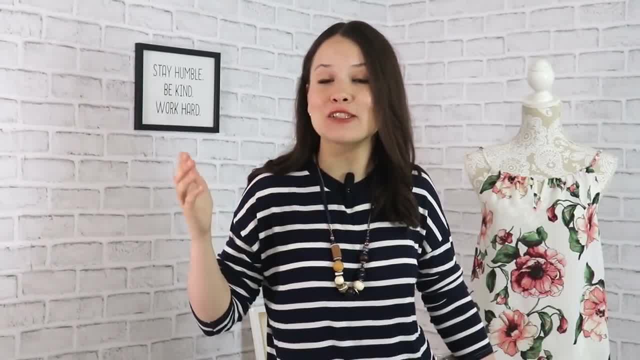 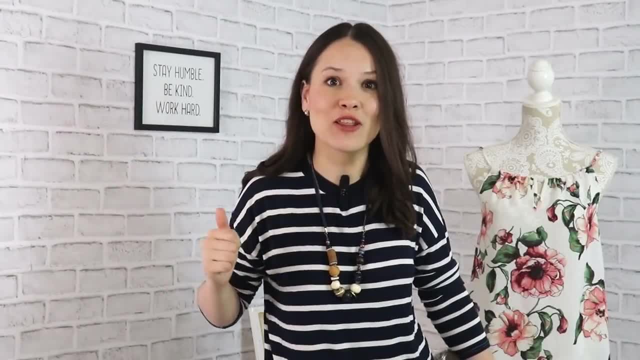 sometime mid-August or at the end of August I am planning another set or about five different items to offer to the local residents towards the start of the school. So that way they have something extra, something new, something to look forward to when they come back to my booth at the farmer's. 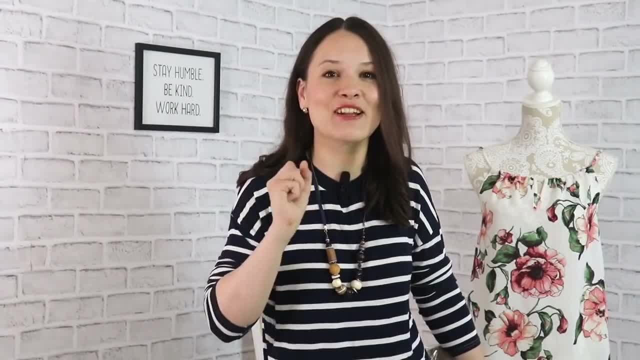 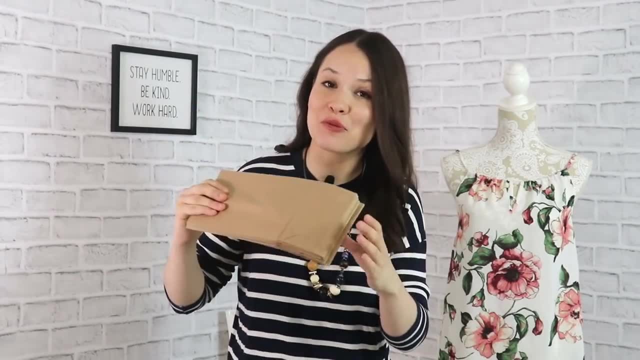 market. So definitely there might be another video with another set of small items to sew and sell at the farmer's market. Bonus idea for you, my dear Starting friends: this is also a really good seller and people absolutely love these. There's. 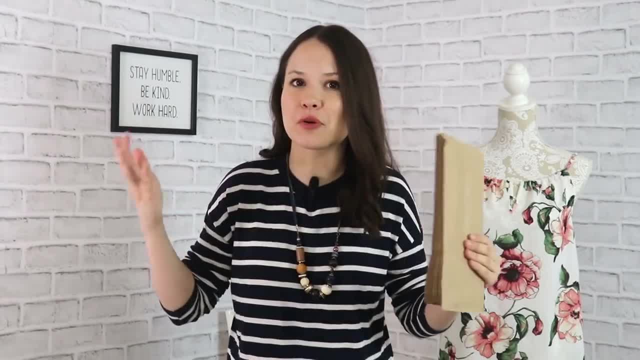 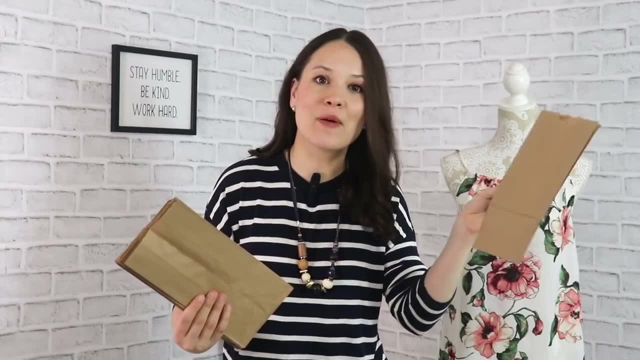 that element of surprise. So what you're going to do is you're going to go to Walmart, Kroger, Dollar Store, Poundland, wherever you are, and you're going to grab these brown lunge bags. They usually come in a pack of hundred and I make about a dozen of these at a time for each week, And I 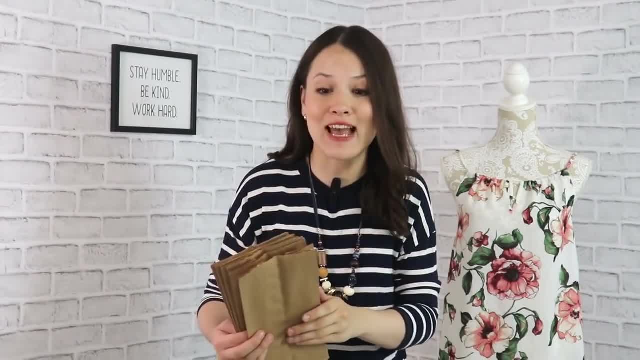 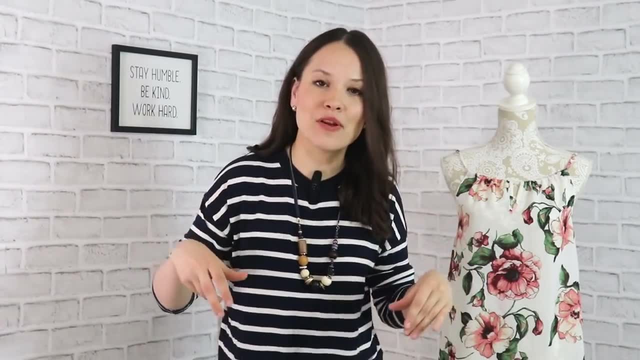 only do farmer's market once a week for four hours on Saturday, So this is definitely a great idea to do. It comes together so quickly too. So what you're going to do is you're going to pop them open And then we call them grab bags. In each of the grab bags, there will be three to four items. One: 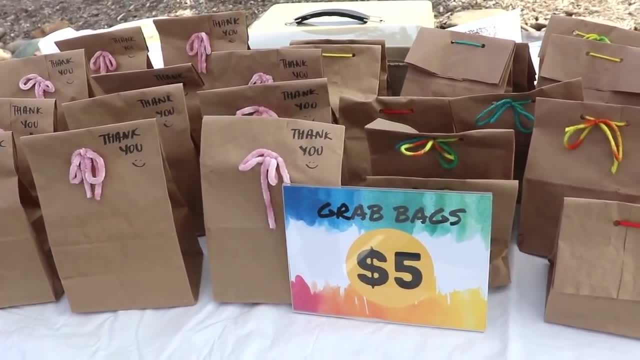 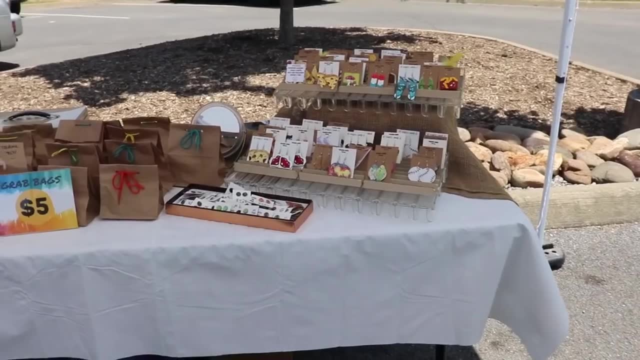 item will be quite a big item, like a scrunchie or a bow or a headband or something like that, And then two additional smaller items that are just fun filler, something for the kids or adults or whatever, And we put them all three items in the bag and then you fold it really nice Sometimes. 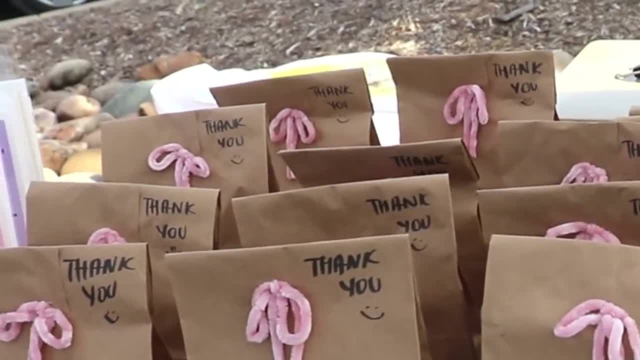 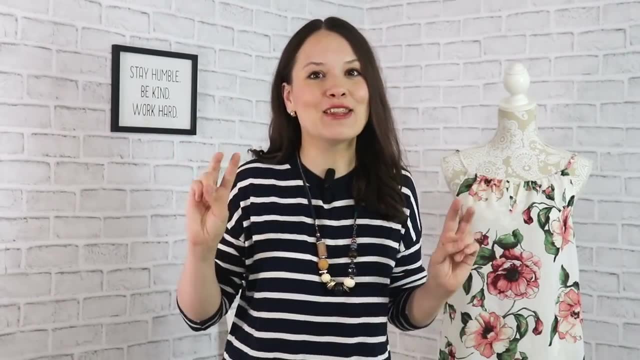 I'll add a little bow that I make from the yard. And then when people come to the farmer's market and they ask what's in the grab bag, What's in the grab bag? And I tell them: well, there's three items. One of them is pretty big, The other two are fun little. 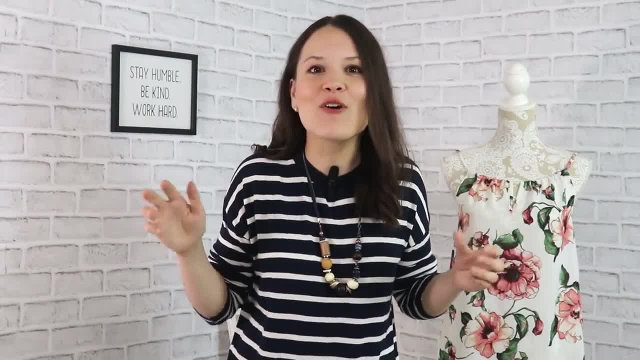 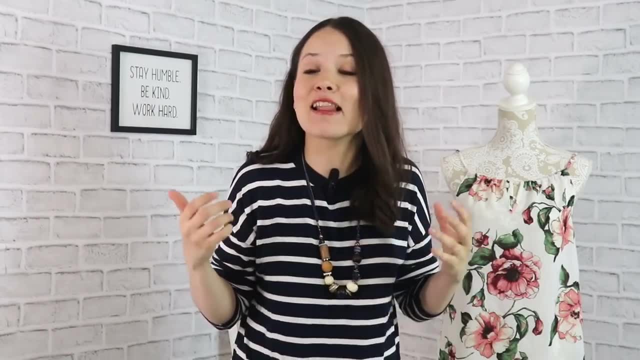 items, additional ones, and you don't know what you're going to get. So a lot of times kids will start shaking them and looking and trying to see what's in the grab bag. It's a lot of fun And a lot of times parents that have kids at home and parents came to the farmer's market to check out. 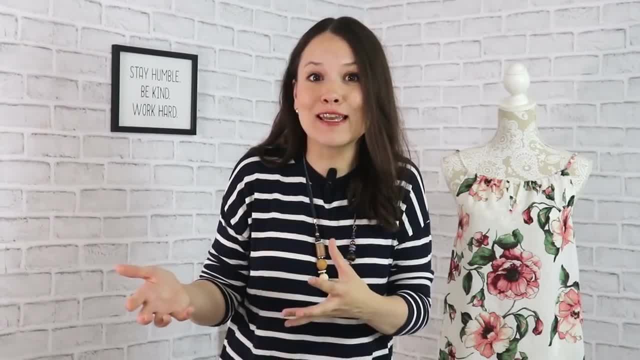 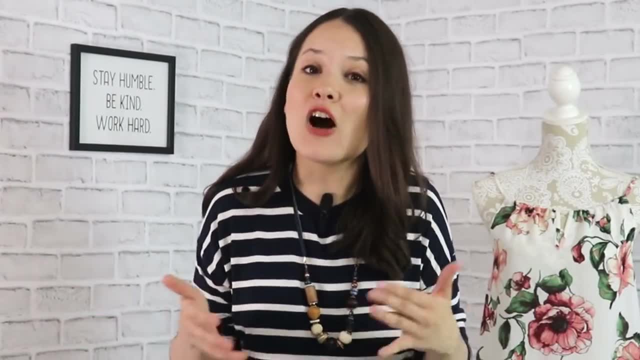 local produce and local crafters. Parents will buy these for their kids as a nice surprise as well, Sometimes on a slower day, let's say a week later- we'll just grab them and they're going to take them. slower day, let's say it's raining- I will only sell maybe four of these. On a good day it's closer to. 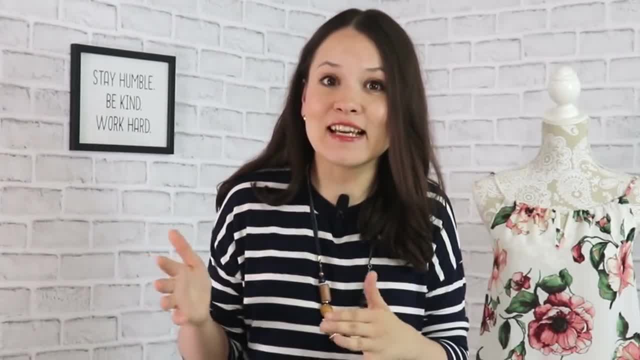 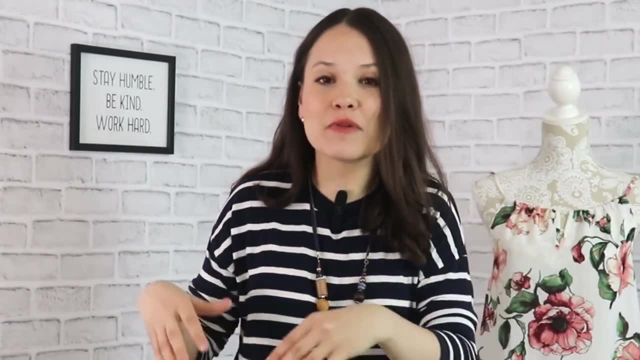 the double digits, so definitely take a look at this idea. This is such a fun, fun activity, and both me and my friend do these with some earrings and some artistic stuff, and for me, of course, this is more of the products that I sell. Therefore, it's really fun to see people get so excited. 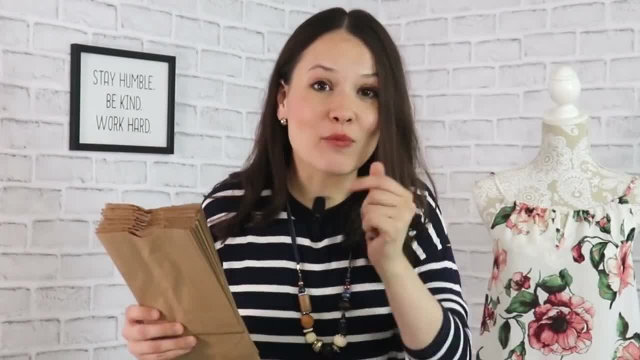 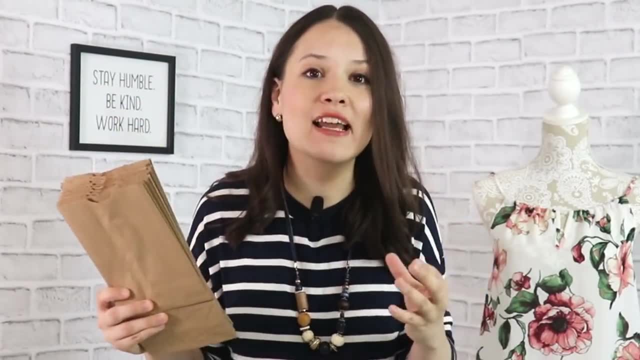 because you don't know what you're gonna get. And on the bright side for you as of the maker of all of these handmade goods, this is a great idea: how to move some of the one-off items that you might have. Maybe you're making things in sets or in collections and you have one or two items that. 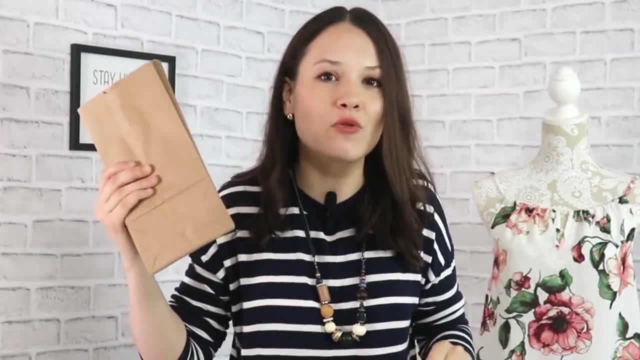 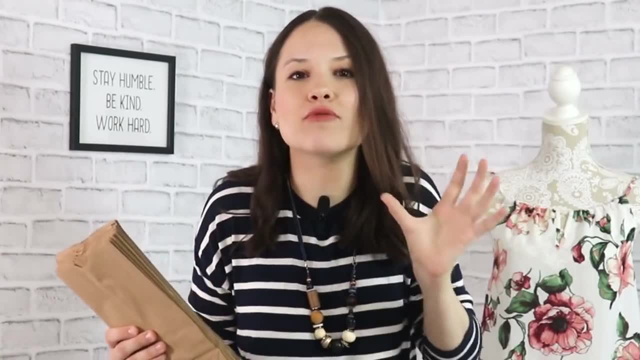 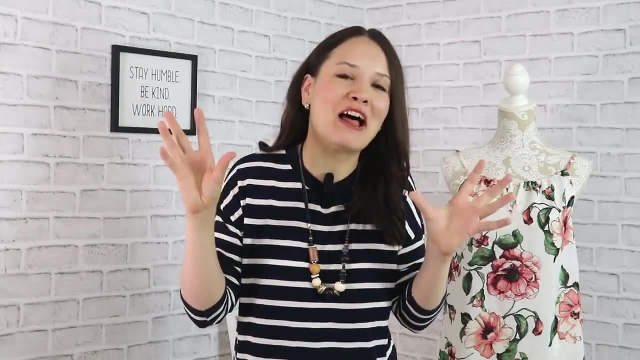 just don't feel right for this or that. This is a really great way how to give people the joy of surprise and also move some of the items that just maybe don't feel right for the collection or color scheme, or maybe patterns or whatever else. Now I gotta tell you, farmer's market is a lot of fun. 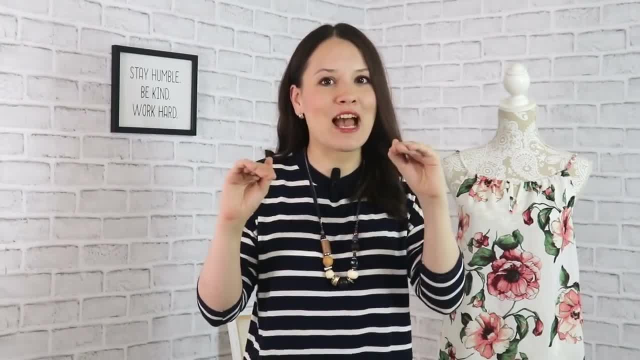 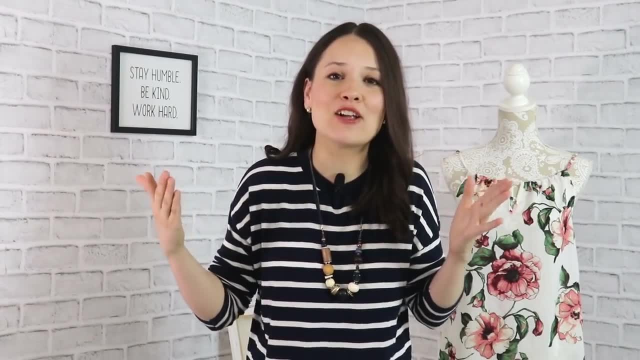 but it's definitely not easy. It has its ups and downs. It's a numbers game. Some days you might do really well, some days you might not do so well at all. But it's really fun to talk to local people, to see what they like, to gain knowledge from them as well. 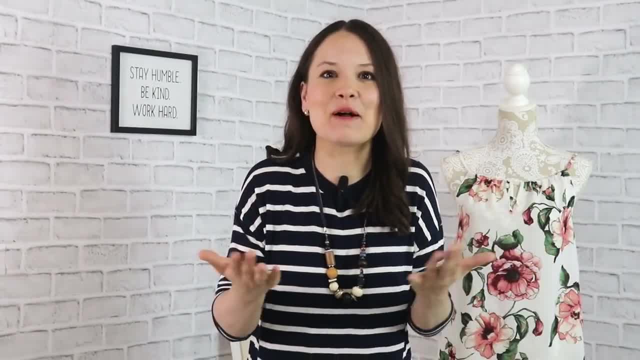 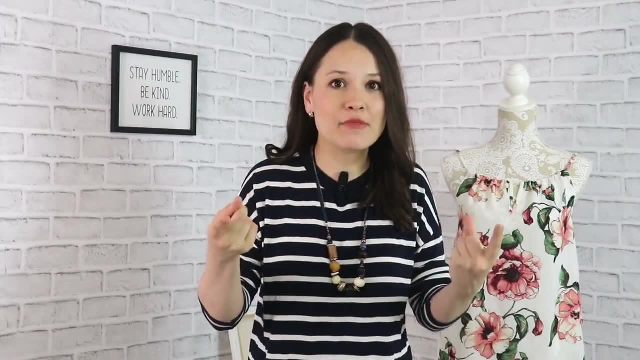 from their suggestions. I get to meet some of my subscribers as well, which is really really amazing And it can be a really great experience. It all depends how you approach it. If you treat it like a business, you will see some success. If you treat it like a hobby, it really just depends on the size. 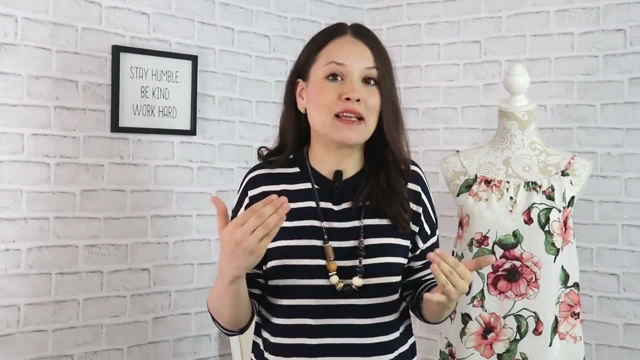 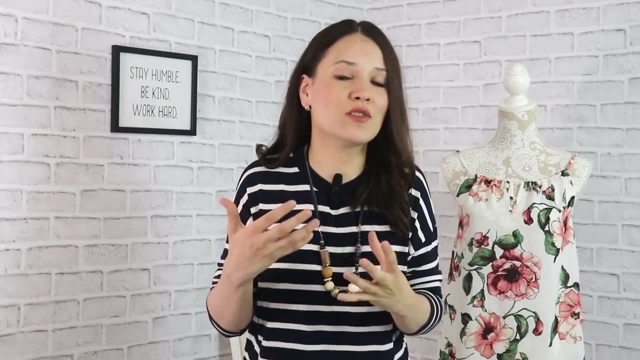 of the farm, How much traffic you get through it and things like that, And what is your expectation all in all? Do you want to make full time living off of it, which might be challenging, or do you want this to be more of a supplemental income?